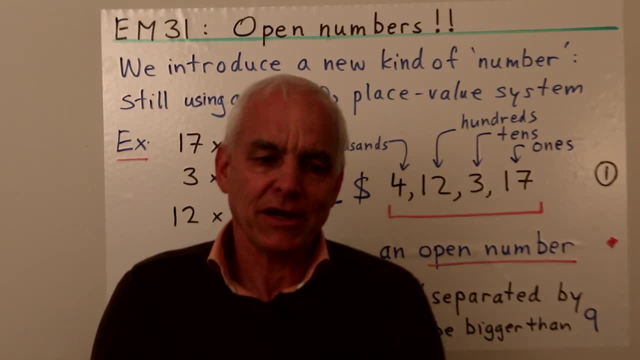 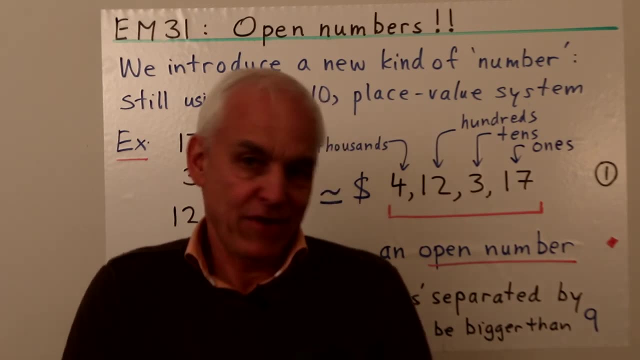 But as I've been doing it, it's been interesting that I've started to realize that when you look at the foundations even of very simple things like fundamental arithmetic, primary school arithmetic, there's insights to be had And there are opportunities for thinking more clearly and more carefully. 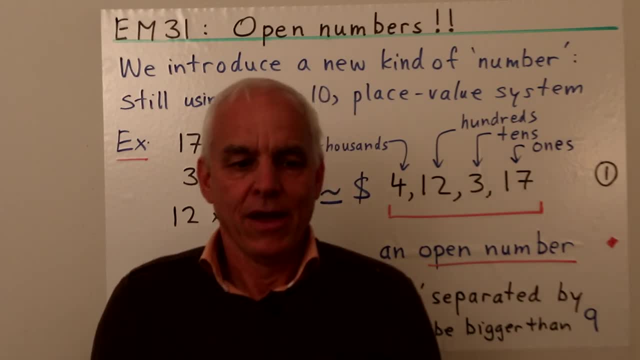 And even in novel directions, And that's sort of what I'm presenting to you now. I'm looking towards re-landscaping this approach. basic arithmetic for young people. I think we can do a lot better than we're currently doing. 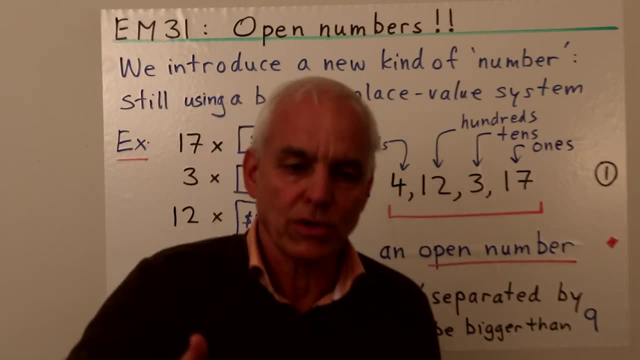 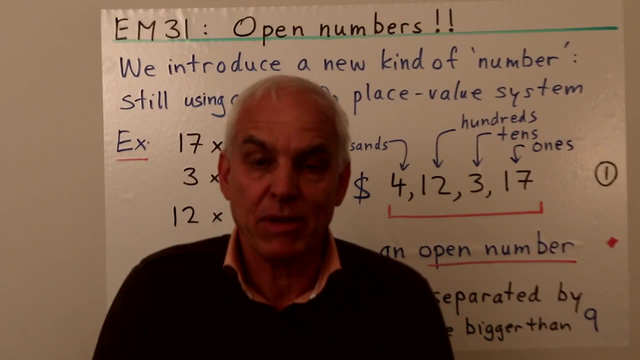 So creating some tools and some notions And some techniques that will actually make it easier for young people to learn how to do arithmetic And to do well, to actually perform calculations more consistently and more correctly. Okay, so a key point here is the introduction of open numbers. 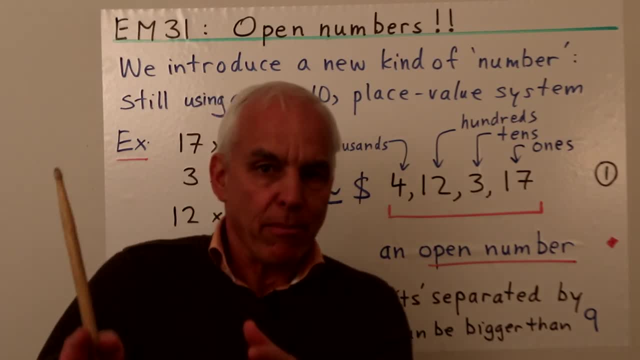 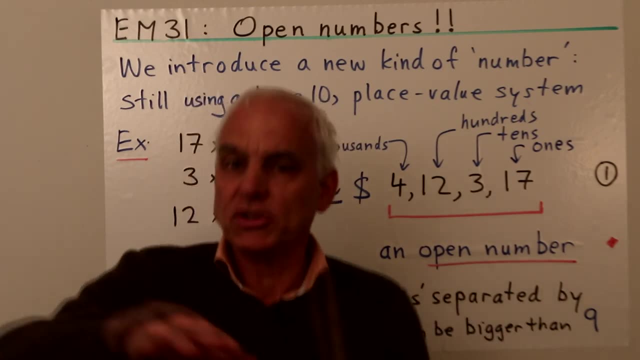 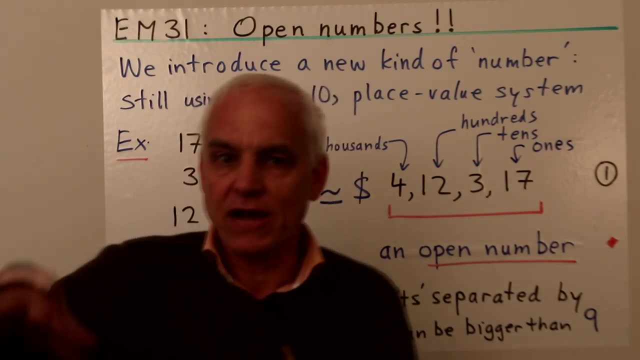 Okay So open numbers are like natural numbers, but a little bit different, And we're sort of augmenting the usual arithmetic by introducing these additional things Which are in some ways simpler to deal with. Okay So we're going to have a simpler kind of arithmetic that will still tie very closely to the usual one. 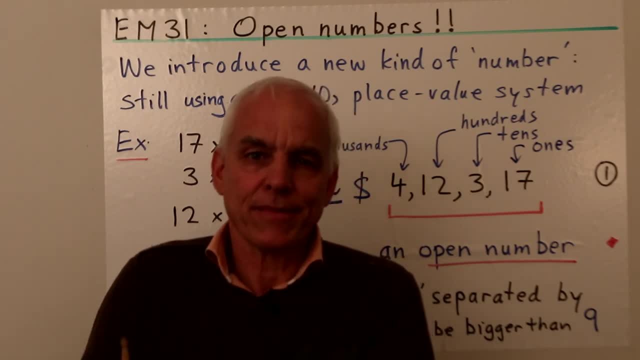 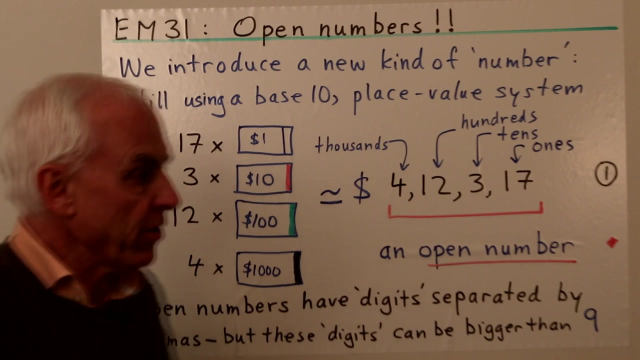 But provides a more enjoyable kind of framework actually to do arithmetic, And it will turn out not just addition, but also addition, subtraction, multiplication and perhaps even division. Okay, So we're going to introduce a new kind of number. 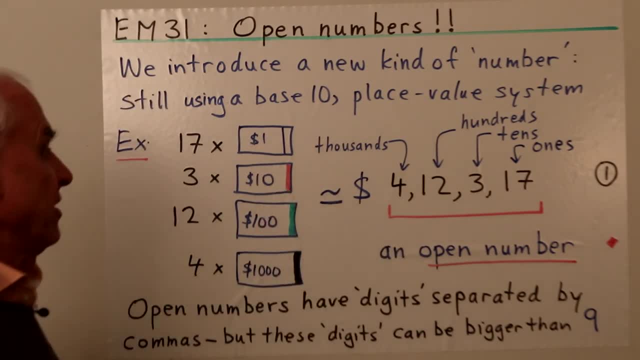 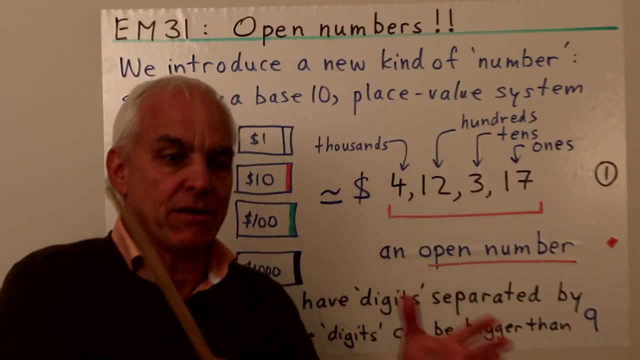 We're still in the base 10 place value And we're motivated very much by money And the usage of money in real life, So having a monopoly set And lots of $1, $2 kind of bills and so on to play with. 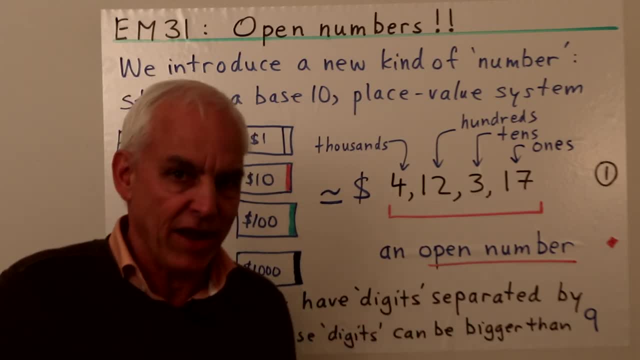 These are great. So we're actually going to only need $1,, $10,, $100, and $1,000.. And the idea is that let's say somebody has this collection of money. They have 17 $1 bills. 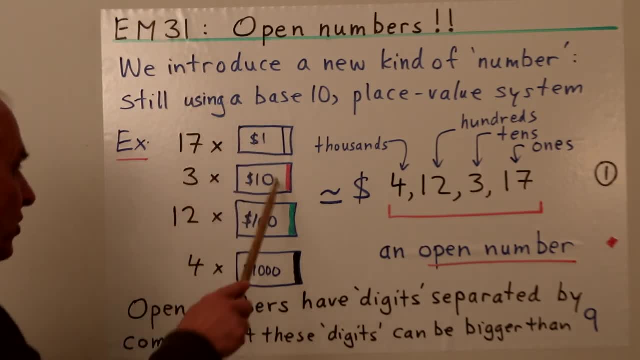 They have 3 $10 bills. They have 3 $10 bills. They have 4 $10 bills. They have 5 $10 bills. They have 6 $10 bills. They have 7 $10 bills. They have 8 $10 bills. 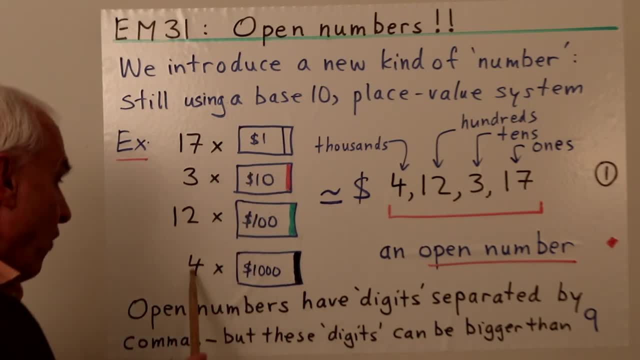 They have 9 $10 bills, They have 12 $100 bills And they have 4 $1,000 bills. Maybe it's monopoly money, It doesn't matter. We want to represent this collection of money, Recording the totals in the various places. 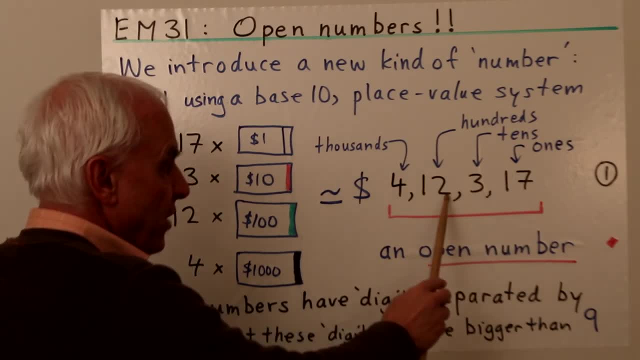 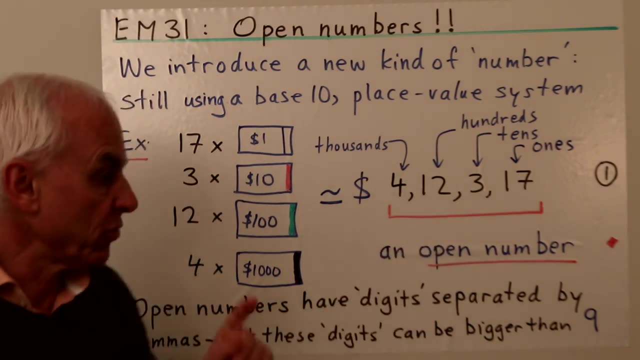 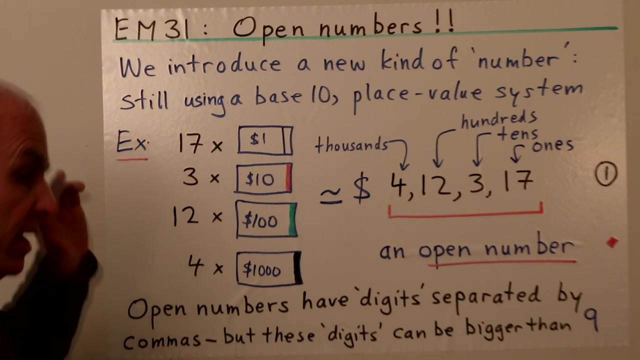 Starting with the ones here, Then the tens, Then the hundreds And the thousands With commas And, crucially, the quantities are any natural numbers written in Hindu Arabic form, But in particular, they can be bigger than 9 if they want to be. 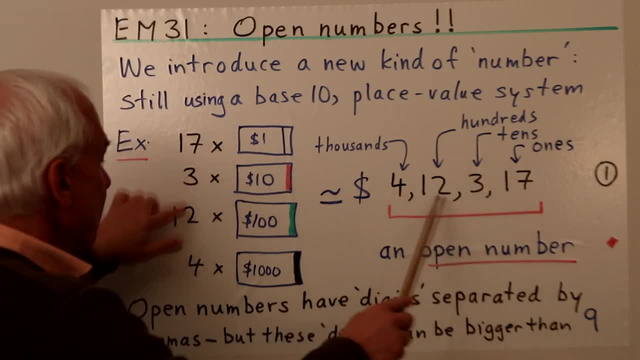 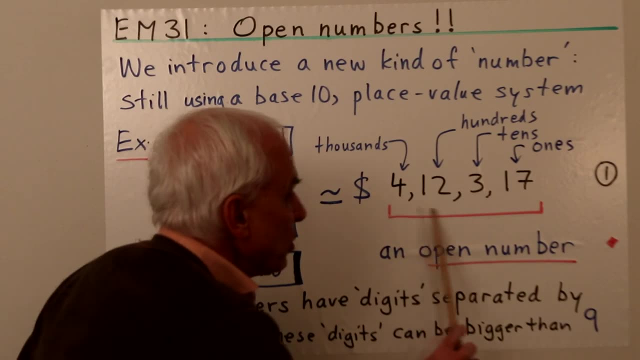 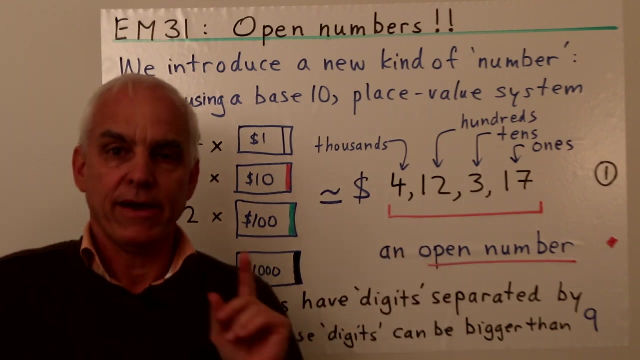 So here we have 17.. 17 ones, 3 tens, 12 hundreds And 4 thousands, And this is all dollars, because we're talking about dollars. But this object right here, Separated by commas, This is what we're going to call an open number. 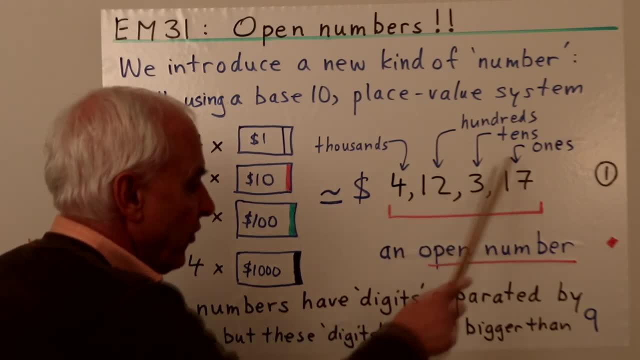 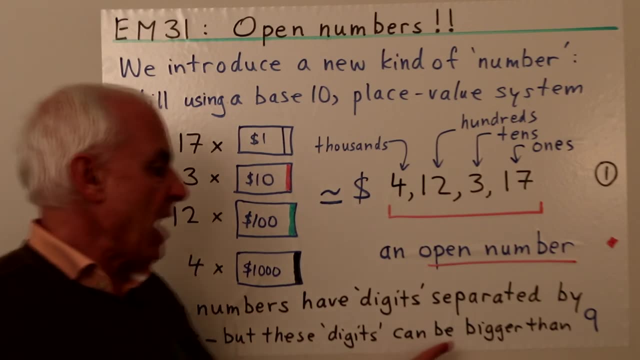 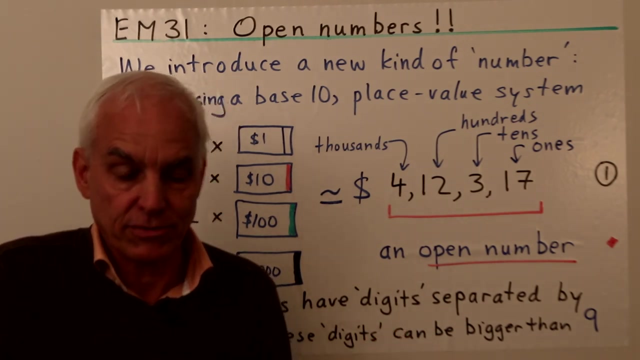 So open numbers have digits Like this one Or this one Or this one, Digits and quotes Which are separated by commas, But these digits can actually be bigger than 9. Like 12. Or 17. Or they could actually be very big numbers. 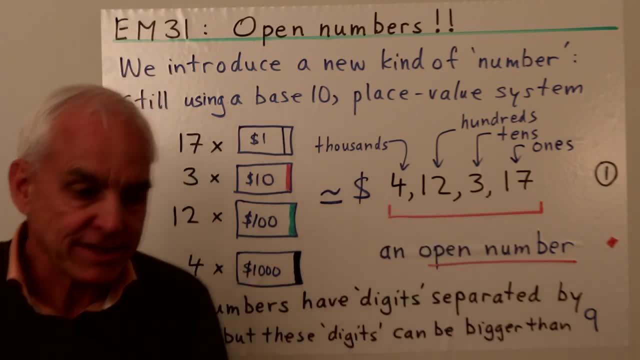 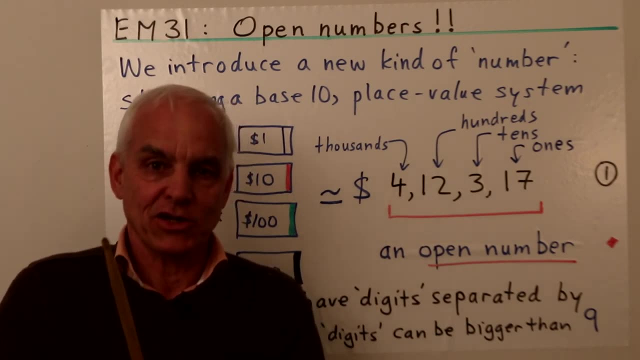 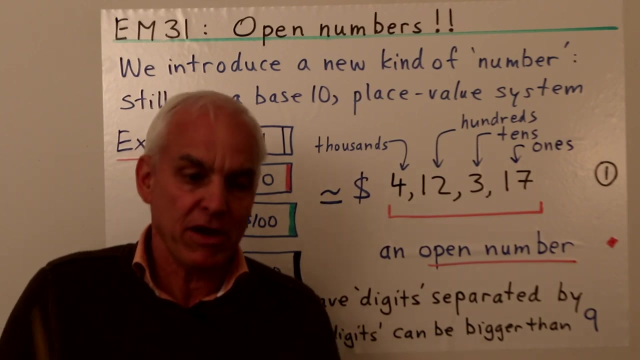 In the thousands or millions. even So, this is an open number And we're going to see that this rather novel kind of number really helps us do arithmetic And helps us explain what's going on with arithmetic to young people. This is a very powerful tool. 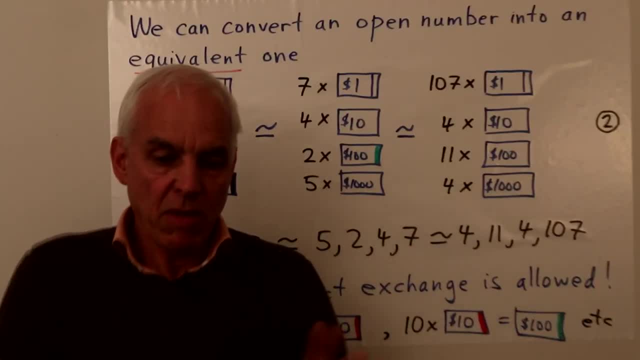 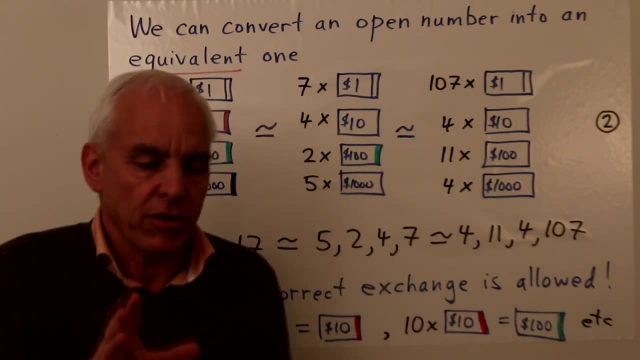 I think Now, if you're a parent or a primary school teacher, you may be thinking: How can you just introduce new kinds of numbers? Is this allowed? Is it legal? Is this really something that we create In order to be able to solve? 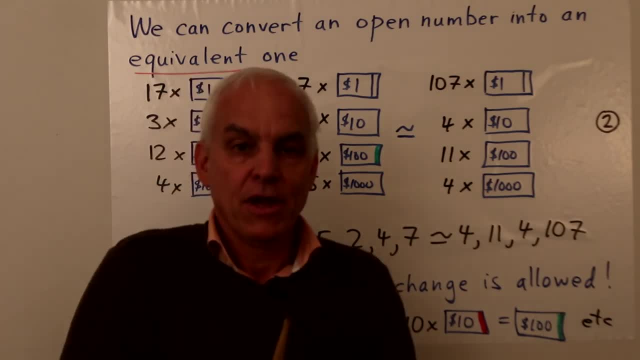 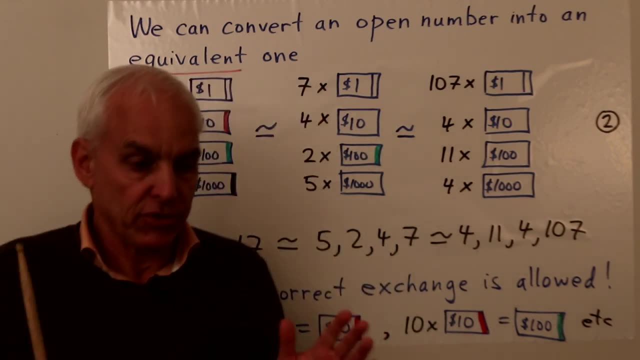 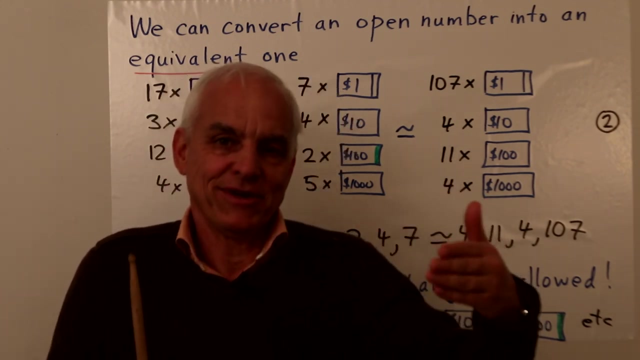 problems in real life, And there are actually many different number systems in mathematics that are used for various purposes, So there's nothing wrong with doing this, But we do have to be a little bit careful that we don't automatically assume things about such a system. 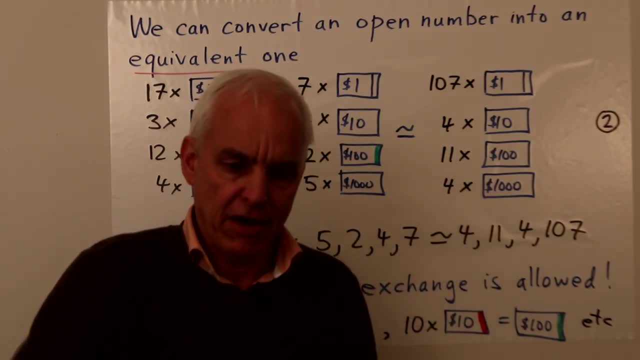 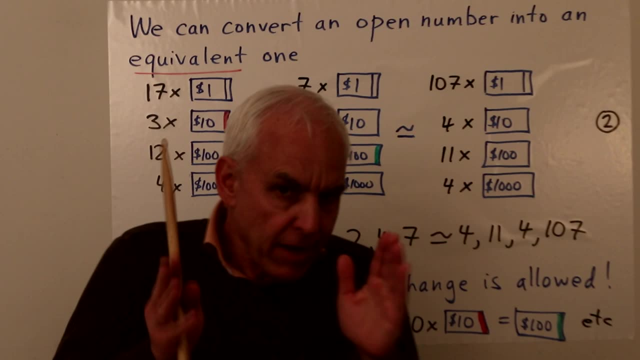 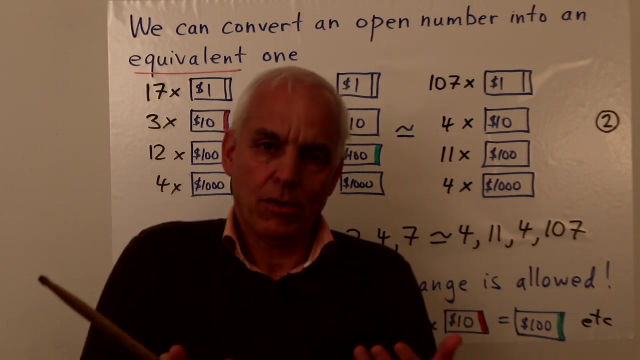 So we are obliged to specify rather carefully various aspects of any new number system. One of the very first things that we need to sort of think about is: when are we going to consider two numbers, whatever they are, equal or equivalent or the same? So in 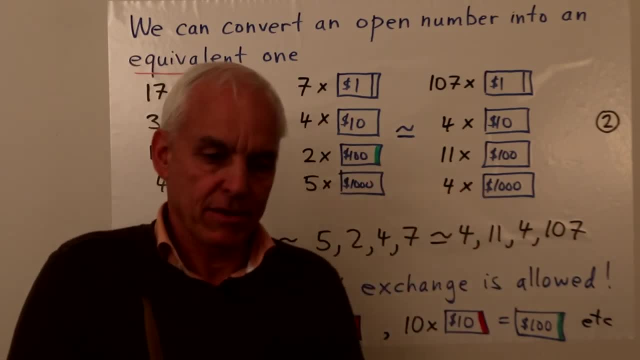 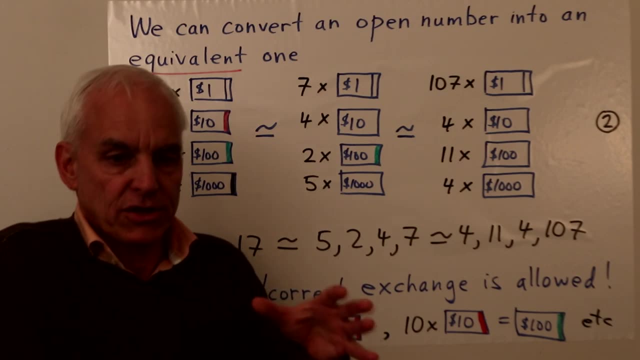 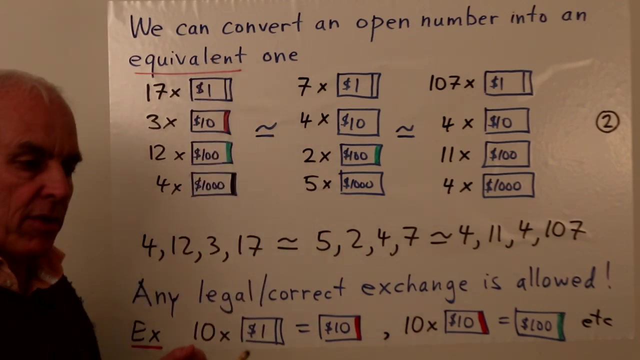 this context, we're motivated by our understanding of money. These open numbers really correspond very closely to collections of bills, And so we're going to introduce a notion of equivalence which is very connected with the notion of equality of money. So we're going to agree that we can convert. 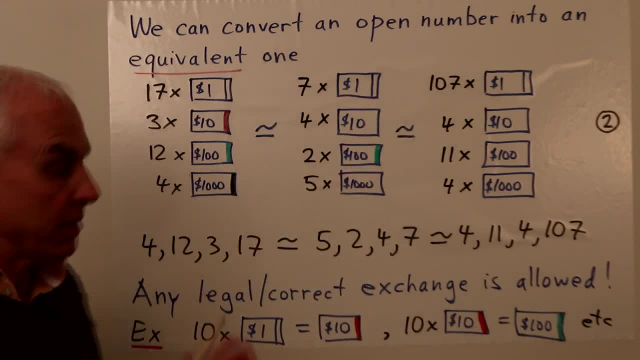 an open number into an equivalent one, And let me show you some examples of that. So here's the same configuration that we started with: 17 one dollar bills, 3 ten dollar bills, 12 hundred dollar bills, 4 thousand dollar bills. 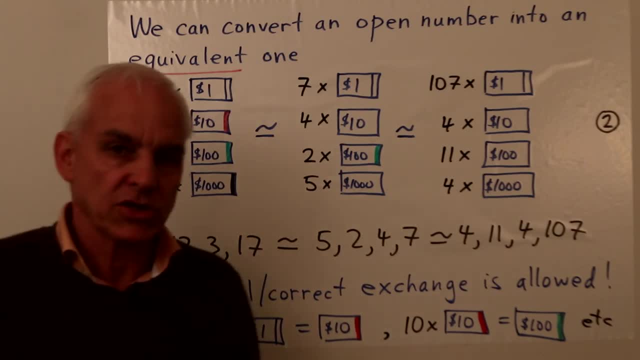 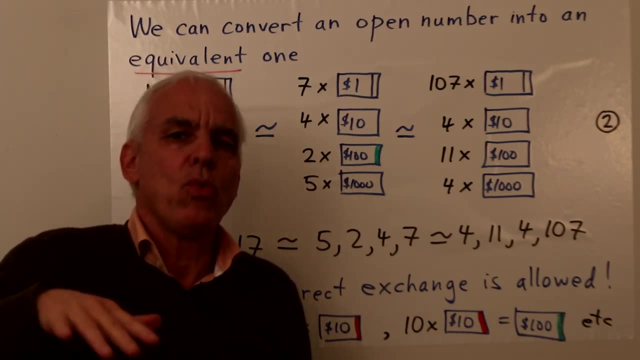 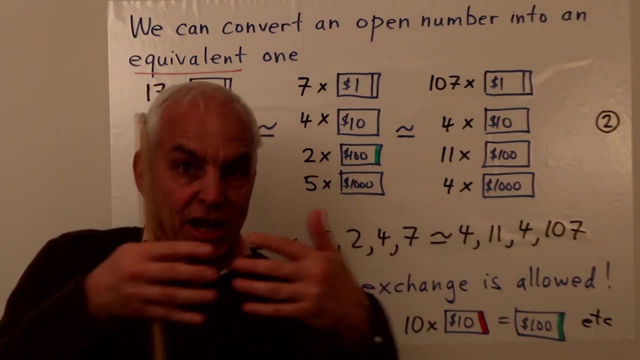 And here I'm introducing this symbol here, which is not exactly equality but rather equivalence. You can think about that as a weaker kind of equality. They're not exactly the same, but they're kind of at the same level. They're very closely connected. 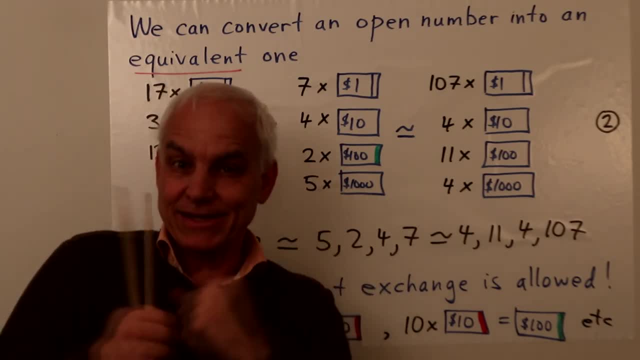 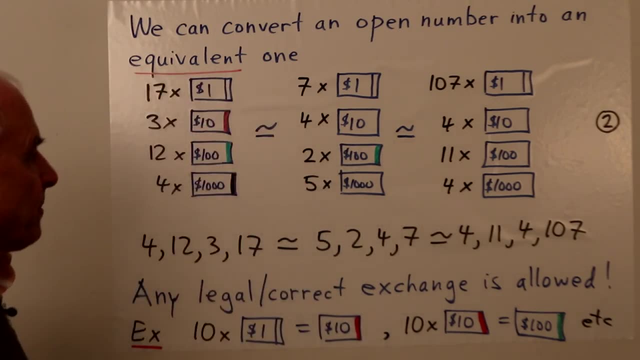 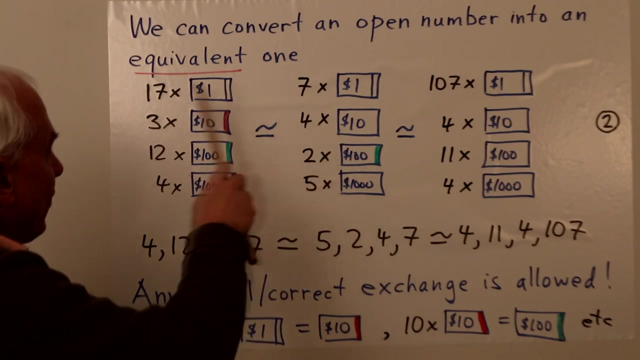 But maybe they have a slightly separate existence still. So that's what this sign means: It's more or less equal, but it's slightly different. And what have we done to go from here to here? Well, we've changed some things. So, instead of having 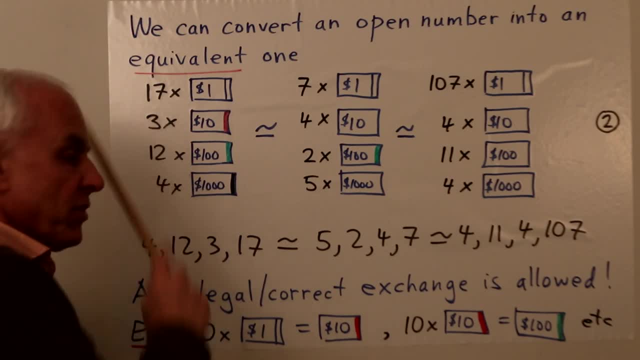 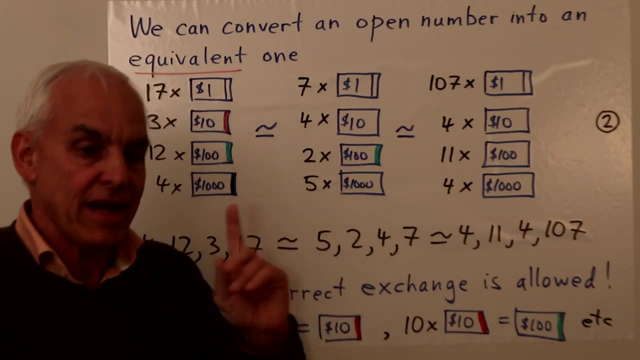 17,. we have 7.. So what happened to the other 10 one dollar bills? Well, we converted those 10 one dollar bills into a single ten dollar bill, And that's why the number of ten dollar bills has increased by one. 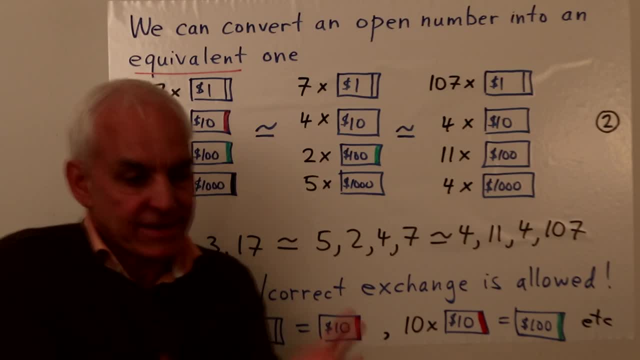 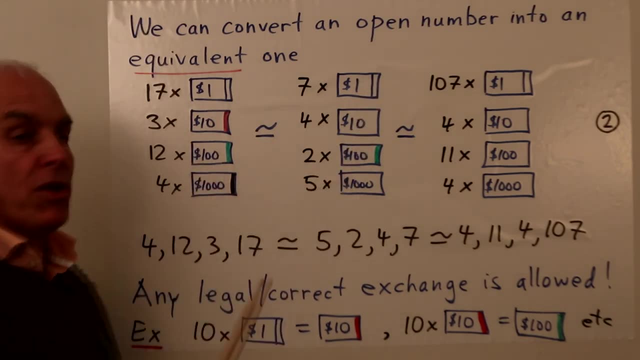 So the total amount of money hasn't changed, but the actual setup, the actual configuration of bills looks different. Instead of having 17 one dollar bills, we have 7 one dollar bills. Instead of having 3 ten dollar bills, we have 4 ten dollar bills. 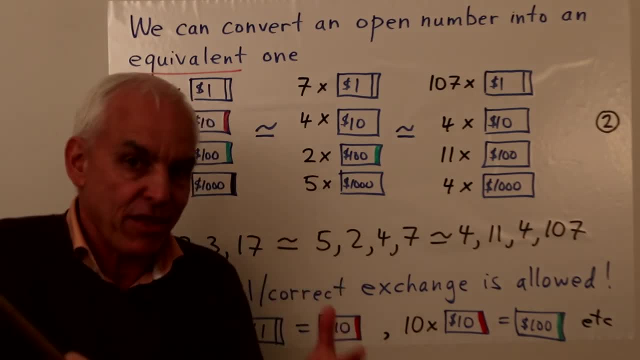 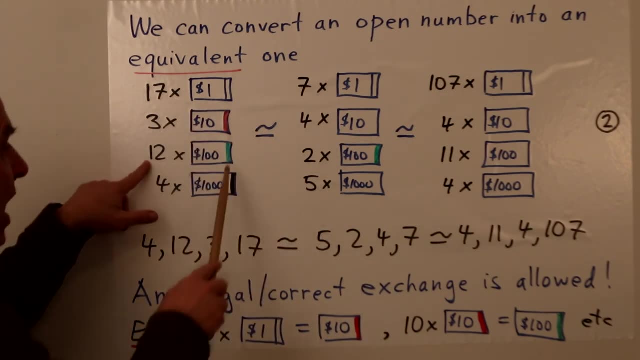 But effectively, in terms of total amount of money, it's the same. So we say that this is equivalent, But we've actually done something else as well. So here there are 1,200 dollar bills, And what we've done is we've taken 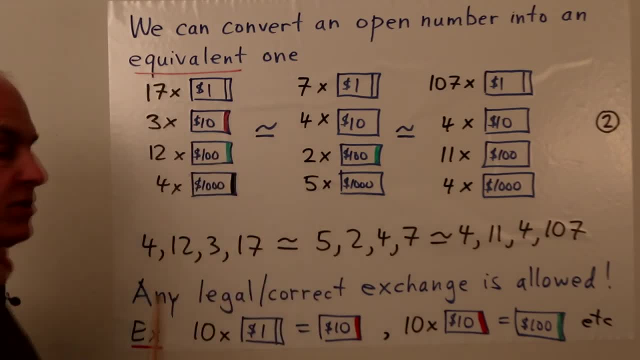 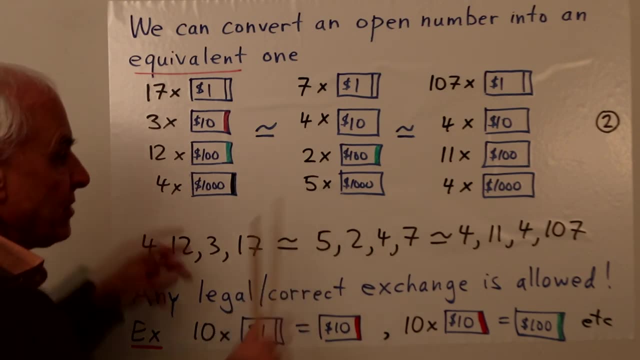 10 of those and replaced them with a single thousand dollar bill. So we have now 200 dollar bills, but the 4 has gone to a 5. We've got 5,000 dollar bills now. I think we'd all agree that this is the same. 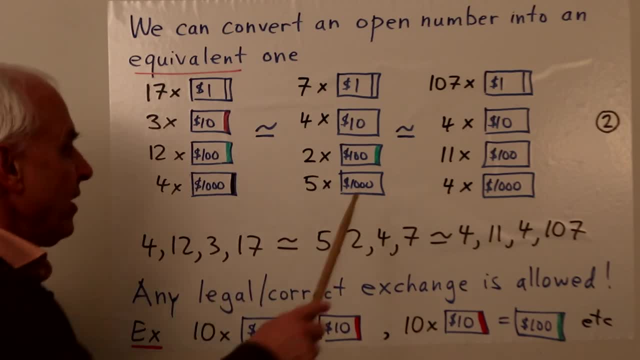 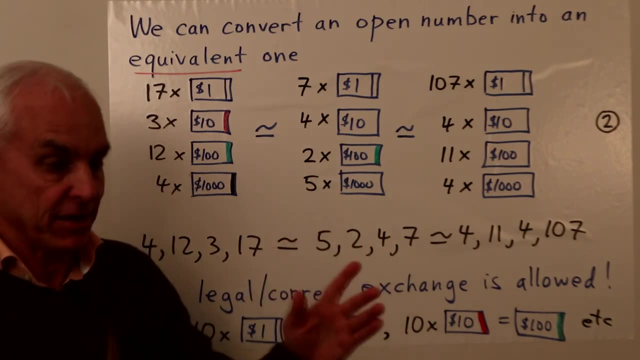 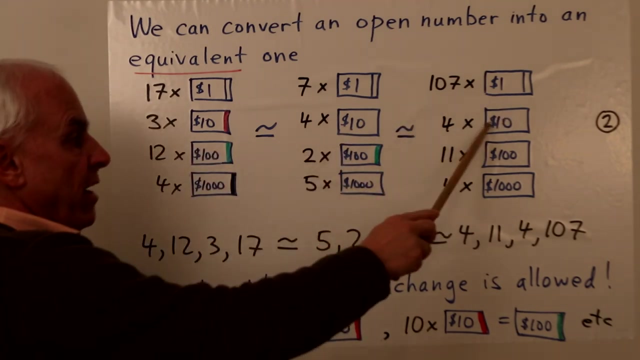 amount of money If you went to a bank and deposited this deposit, and this deposit are going to end up increasing your bank account by exactly the same amount. What about going from here to here? Now we have 107 ones. Still 4 tens. 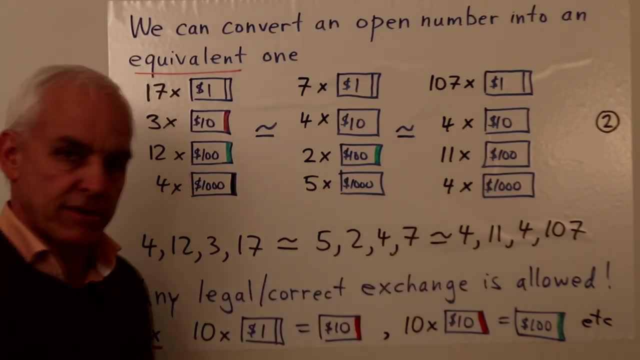 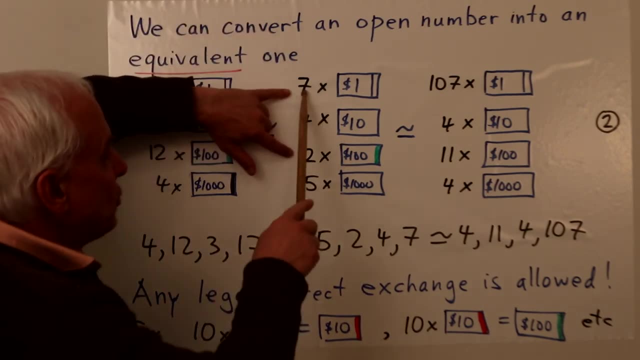 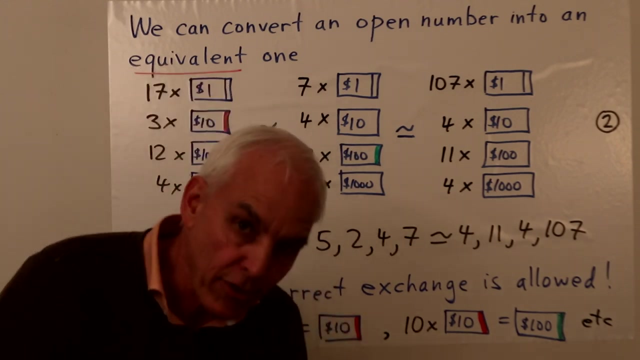 11 hundreds and 4 thousands. Okay, why are these two equal? What's happened here? Well, what we've done to get the 107 is we've taken a 100 dollar bill and we've cashed it into 100. 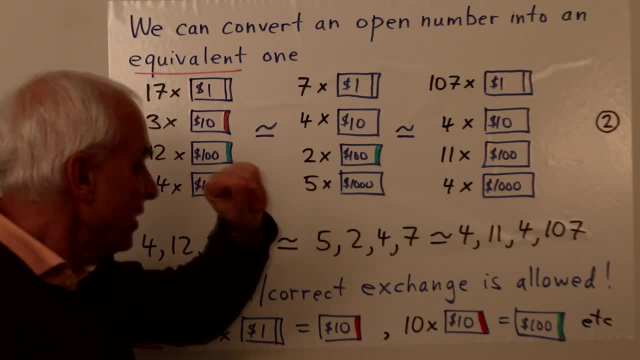 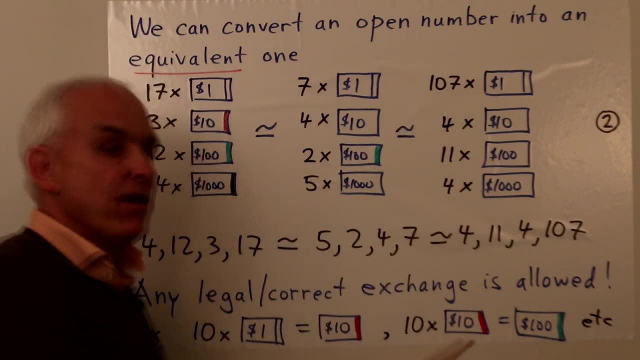 one dollar bills. So imagine taking one of these 100 dollar bills and exchanging it for 100 one dollar bills, to give a total of 107 one dollar bills. There will still be 4 10 dollar bills, but now there will be instead of having 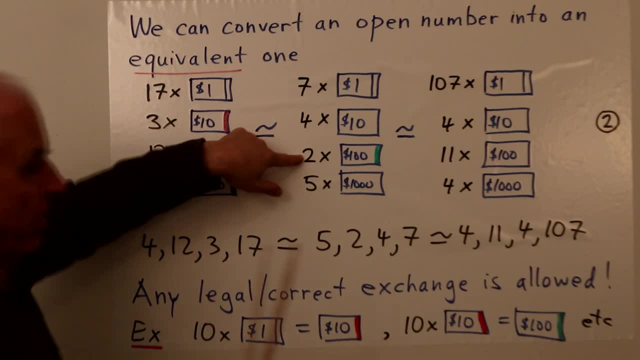 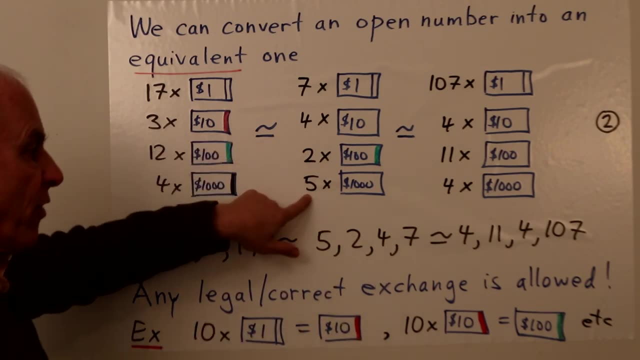 2, there will be 1 hundred dollar bill. But wait a minute, now we have 11.. Where did the 11 come from? Well, we got 10 more 100 dollar bills by converting a 1 thousand dollar bill into hundreds. 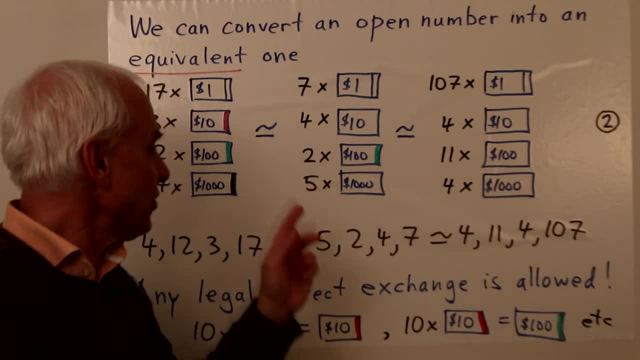 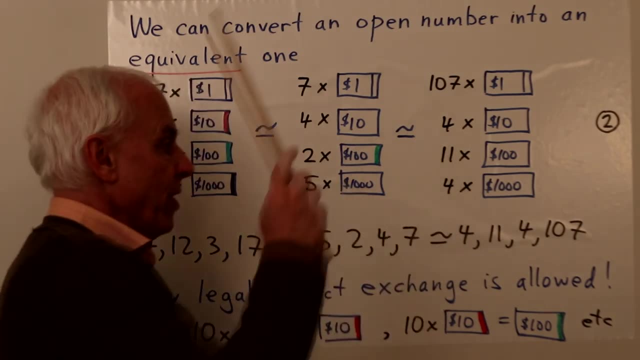 1 thousand is equal to 10 hundreds, So instead of having 5 thousands, we have 4 thousands. One of them was converted into hundreds, And that's why we have 11 there. Now we can express the same thing without drawing. 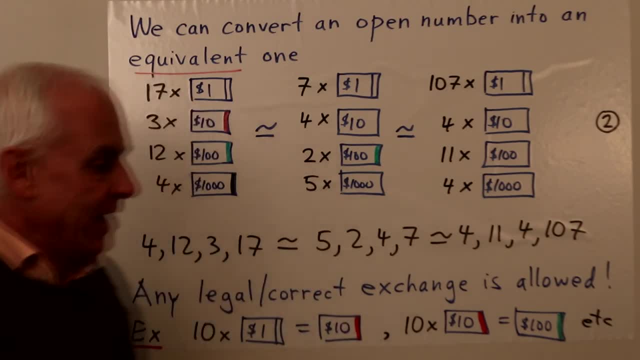 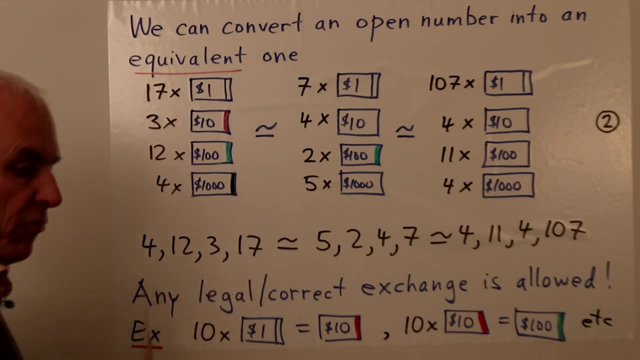 pictures with lots of dollar bills and so on as open numbers. This thing here represents the open number 17, 3,, 12,, 4,, reading from right to left, starting with ones, then tens, hundreds and then thousands Over here we have 7,. 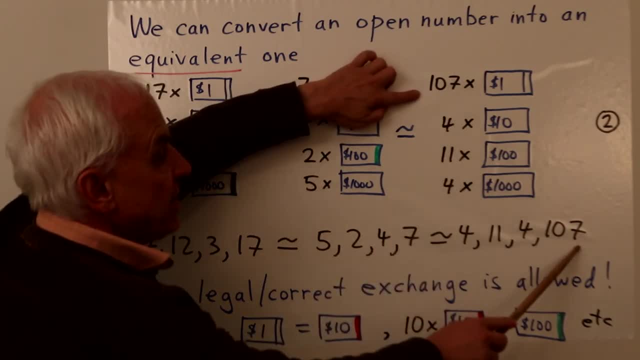 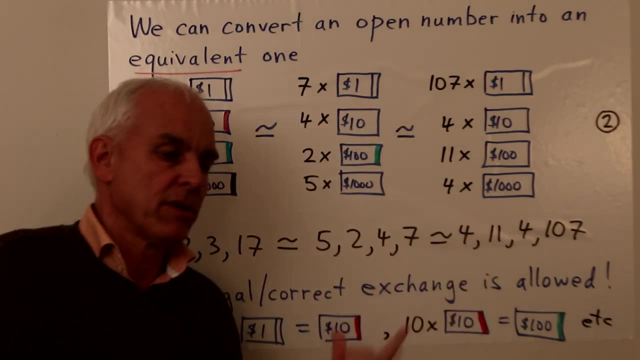 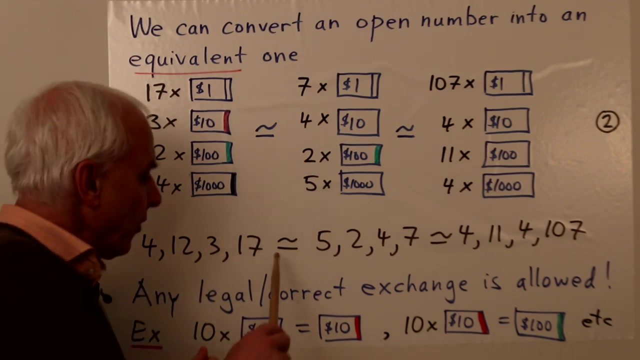 4,, 2, and 5. And over here 107,, 4,, 11, and 4.. And we say that each of these open numbers are equivalent, represented with this kind of equality sign. So a straight bar at the bottom and a 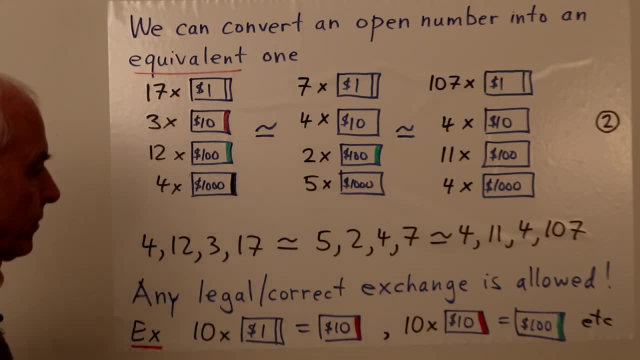 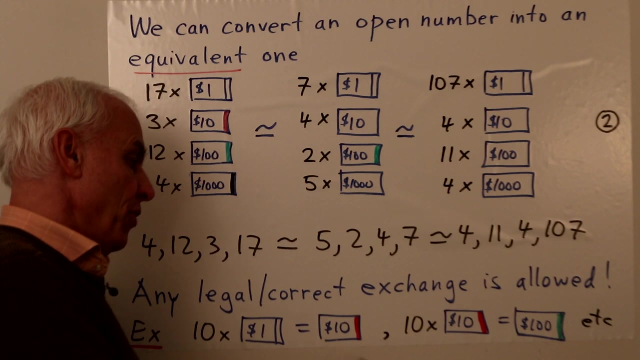 wavy bar at the top. So to go from an open number to an equivalent one, any legal or correct exchange is allowed. By that I mean we're allowed to replace 10 one dollars with a ten dollar, or replace 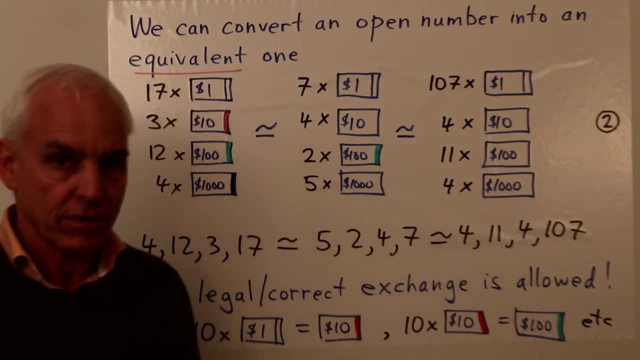 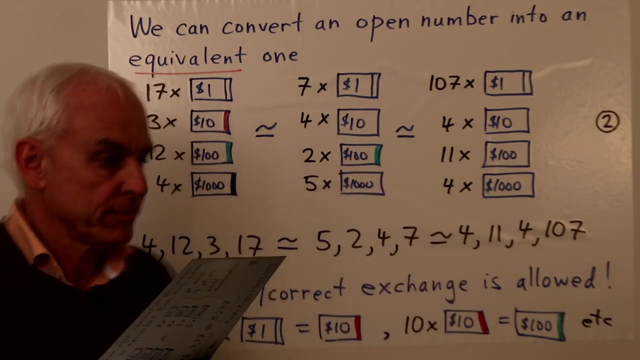 10, ten dollars with a hundred dollar, etc. So there's actually quite a lot of different configurations that we could replace a given open number with To get an equivalent open number. Now, a very important type of conversion is to convert an open number into: 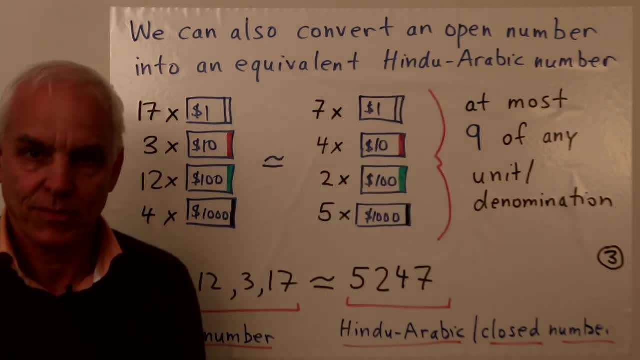 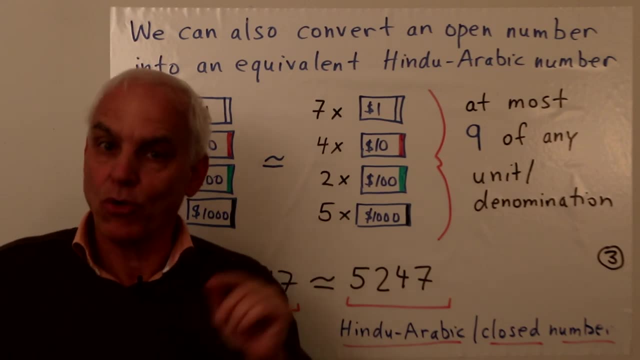 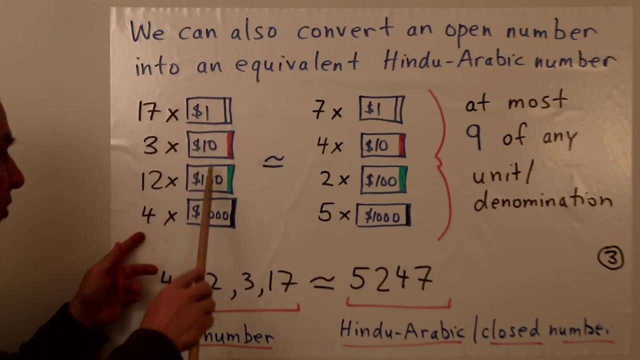 an equivalent Hindu Arabic number. I remind you, that's a number where all the coefficients or all the entries or digits are numbers between 0 and 9.. So, for example, going back to our situation, 17 ones, 3 tens, 12 hundreds. 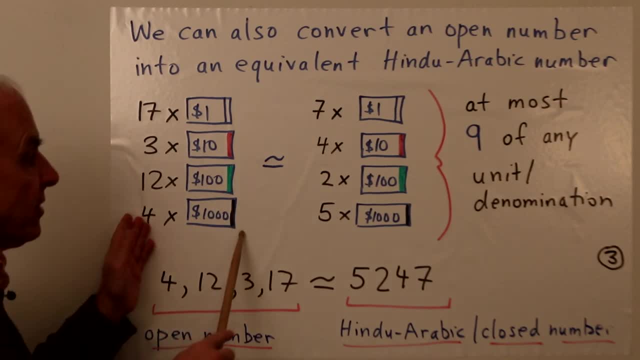 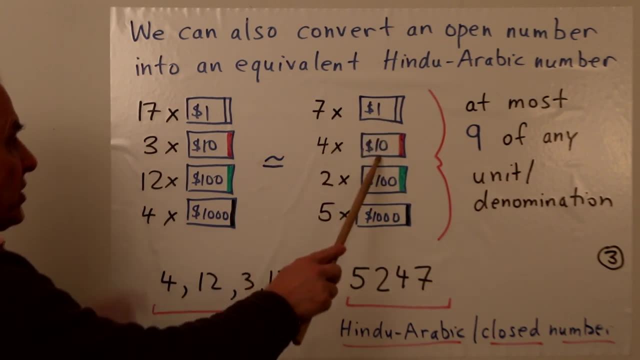 and 4 thousands. we can convert that into this: 7 one dollars, 4 ten dollars. so we've taken 10 of the ones here and exchanged for a 10, 2 hundreds. what we've done is we've taken 10 hundreds and converted. 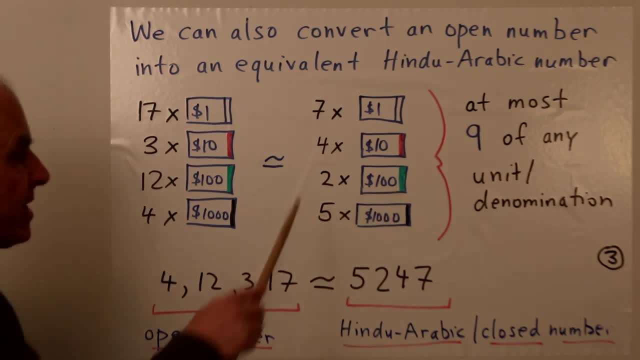 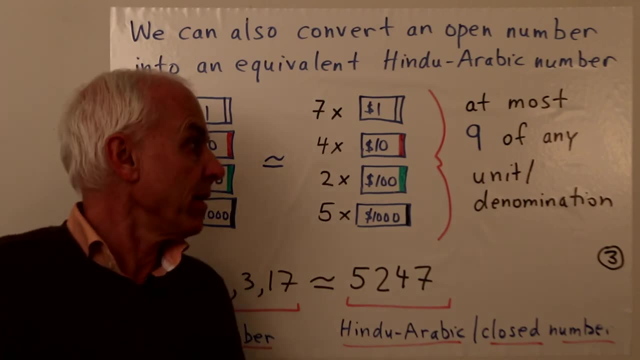 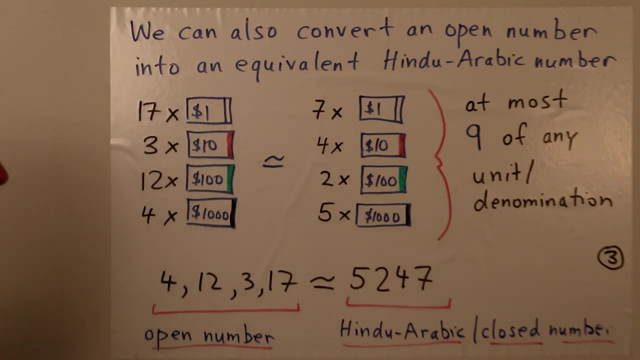 it into a thousand to get 5 thousand. Now the numbers of each bill is a number between 0 and 9.. So there's at most 9 of any unit or denomination. This is what characterizes a Hindu Arabic number. Otherwise they're really pretty. 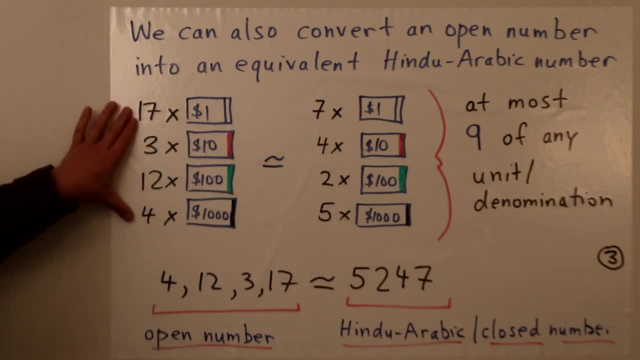 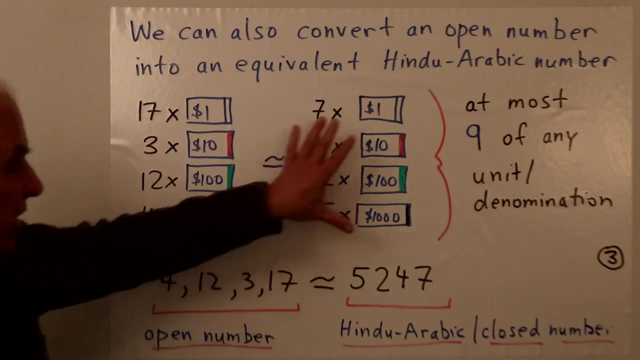 well, the same as open numbers. So we've established that this open number here, 412317, is actually equivalent to the Hindu, Arabic or usual number 5247.. The advantage in this system here is that there's always exactly one way of representing a number. 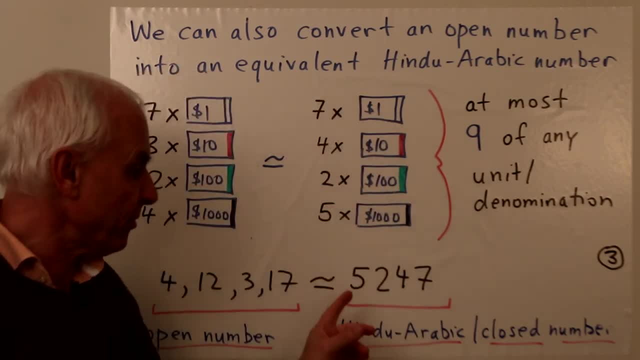 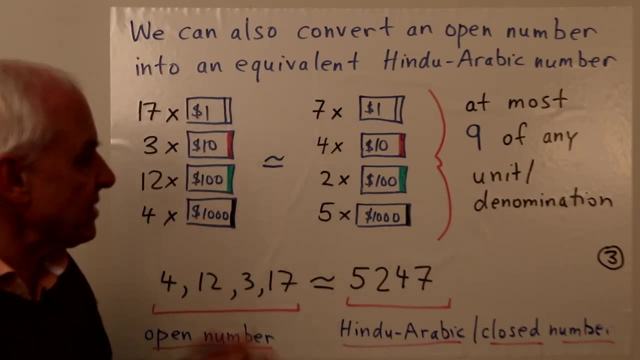 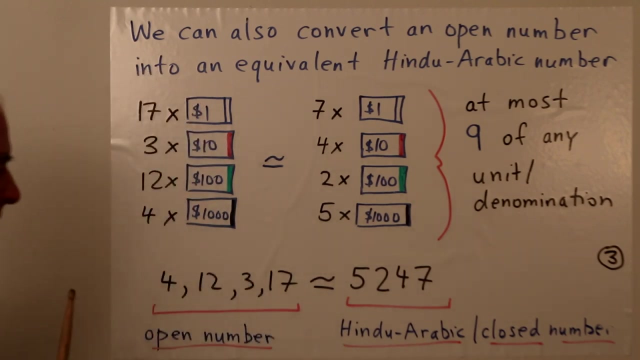 There's no alternative ways of representing this Hindu Arabic number as a Hindu Arabic number, But the price for that is that we have to fuss around to get the coefficients in exactly the range required. So there's actually benefits for both of them, of course. of course, there's lots of benefits for this. 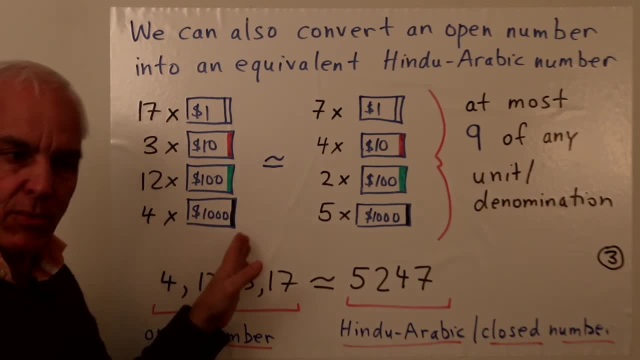 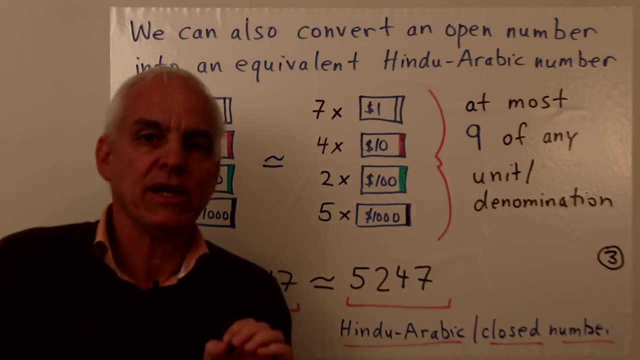 But it turns out there's also benefits from this point of view, that we gain something in certain situations by having this more flexible point of view, And it turns out that's exactly what we need to do: a lot of primary school arithmetic, So there's lots of exercises. 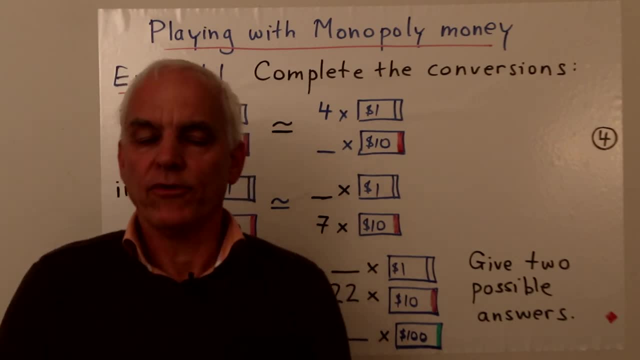 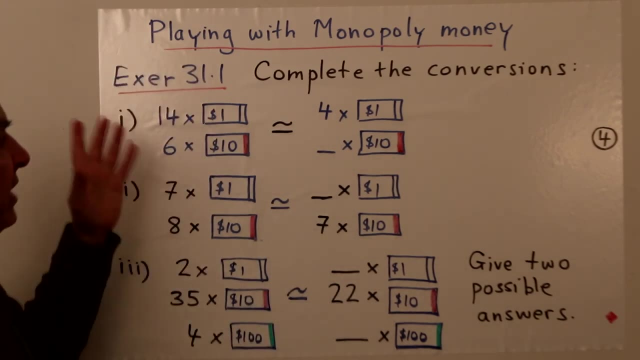 that we can now do to get used to open numbers and a little bit of how they work, especially with respect to conversions. So, for example, have a look at this. We're asked to complete the conversions. Here's an open number, here's another. 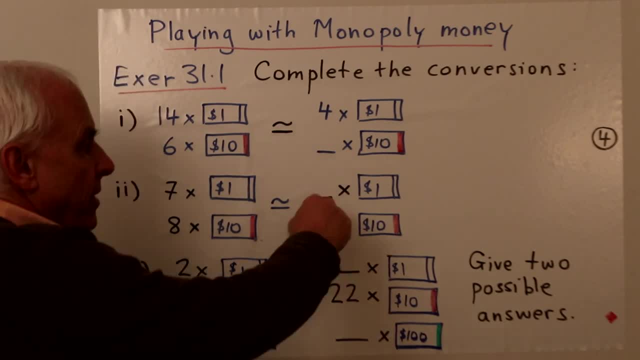 open number, but we have to figure out what that coefficient is there, or how many tens there are. Okay, so here we have fourteen ones and six tens, and over here we have four ones. How many tens do we have? Well, to go from here to here. 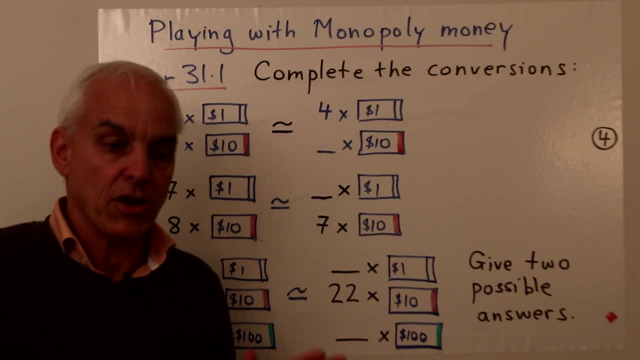 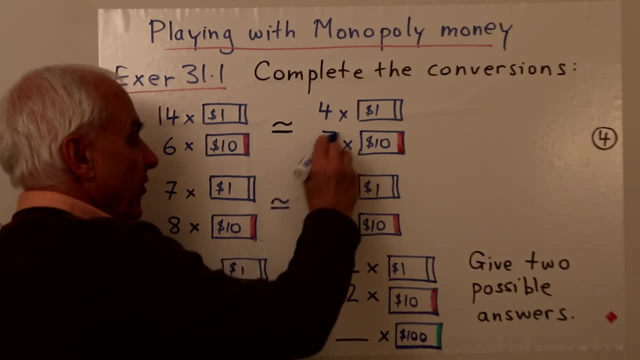 we've lost ten ones. The ten one dollar bills have been converted, obviously, into a ten dollar bill, so there's one more ten dollar bill than there was earlier. There must be seven ten dollar bills Over here. there's seven one dollar bills. 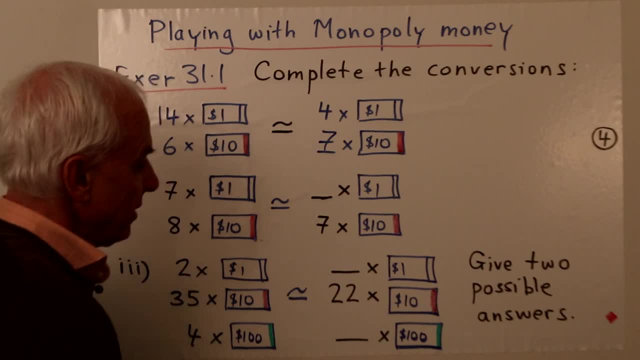 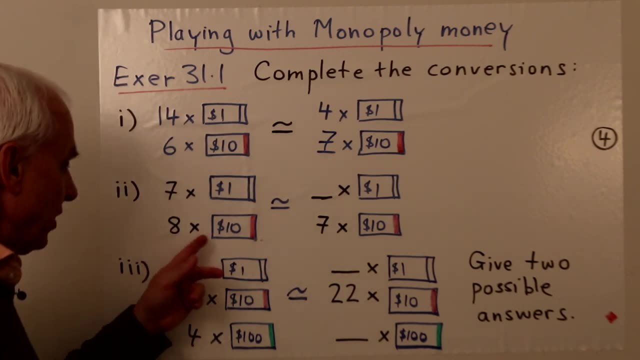 eight, ten dollar bills, and over here we see that there's seven ten dollar bills and we want to know how many one dollar bills are there. So in this case we've taken one of the ten dollar bills and converted it into a certain number of one dollar bills. 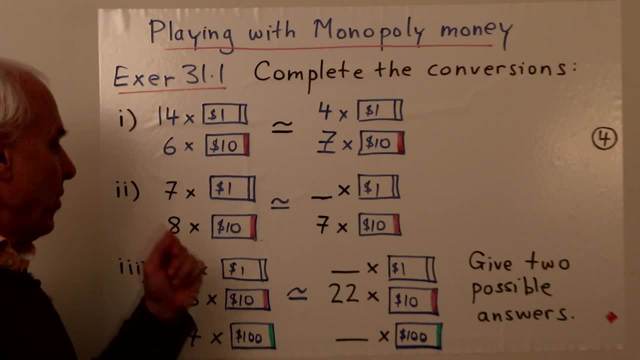 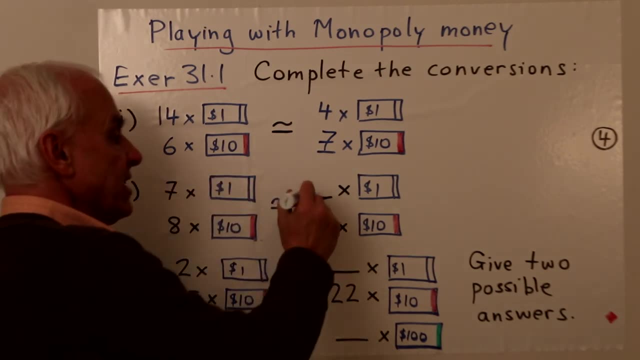 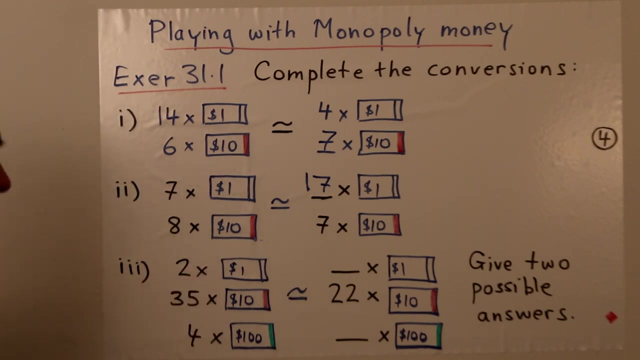 In fact ten of them. So we have seven to begin with. we add ten more because of this conversion of the ten dollar bill. so we must have seventeen up here Here. two one dollar bills, thirty-five ten dollar bills. 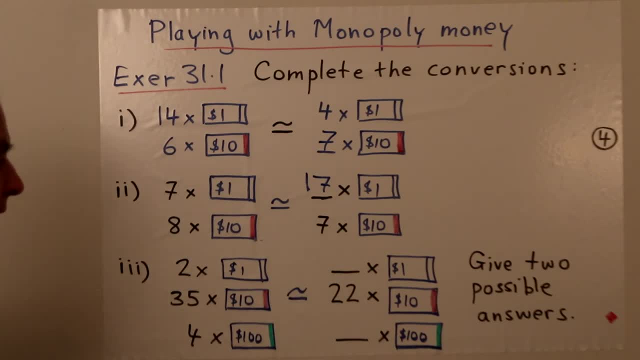 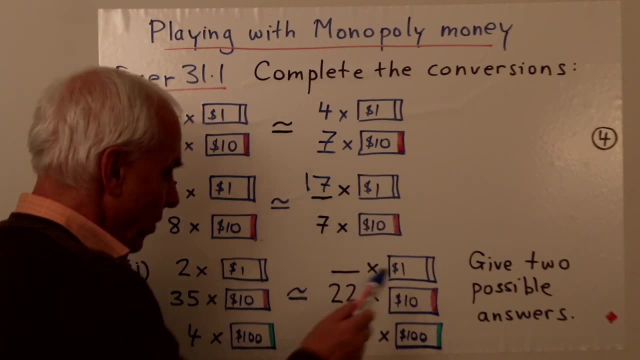 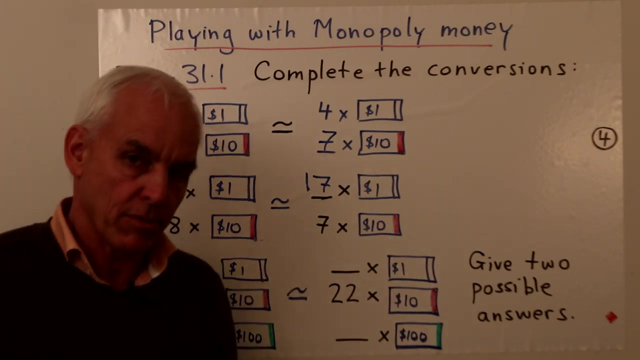 and four hundred dollar bills, And over here we have. well, there's two blanks and we're told that there's twenty-two ten dollar bills. Now there's actually maybe more than one possible answer here, so let's find at least one answer. 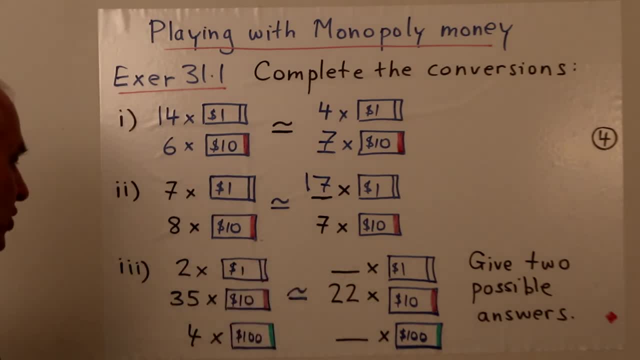 and I'll let you have a look for some other ones. So we're going from thirty-five tens to twenty-two tens. So how could we change tens? Well, we could take ten of them and make a hundred, Okay. so if we 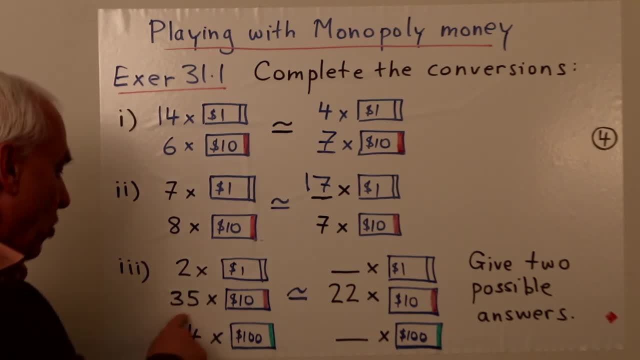 took ten of the ten dollar bills, that would make a hundred. That would then lower us to twenty-five. Okay, so let's actually do that. That's a good step. So we're going to convert ten of these to hundreds giving. 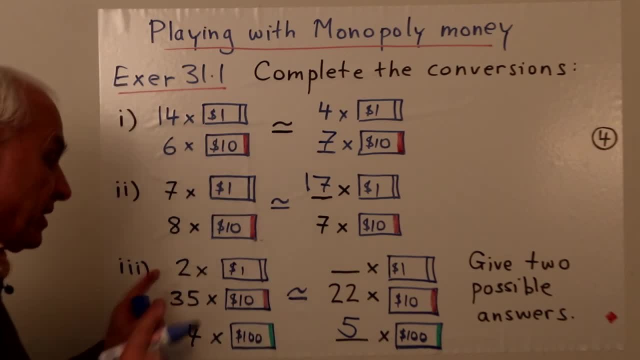 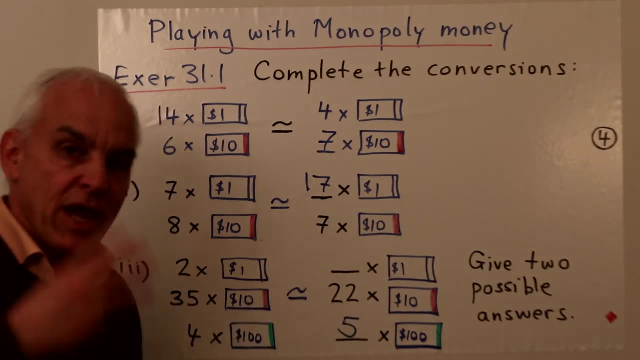 us five hundreds all together over here Now. at this stage we still have twenty-five ten dollar bills and we want to ultimately have twenty-two of them. That means we have to get three ten dollar bills converted to one dollar bills. Three ten dollar bills. 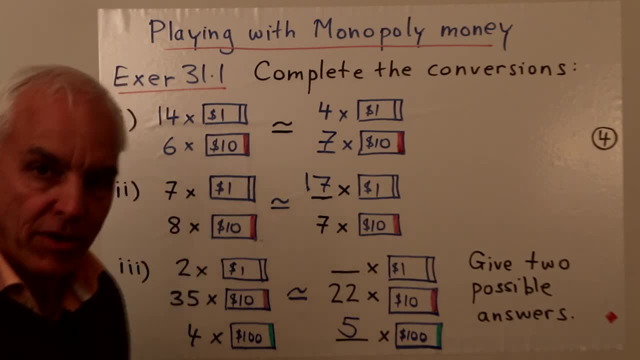 makes ten, twenty thirty one dollar bills. Actually, that's a calculation that everybody knows, right. Three ten dollar bills is the same as thirty-one dollar bills, So we started with two one dollar bills. we've got thirty more, so we should have thirty. 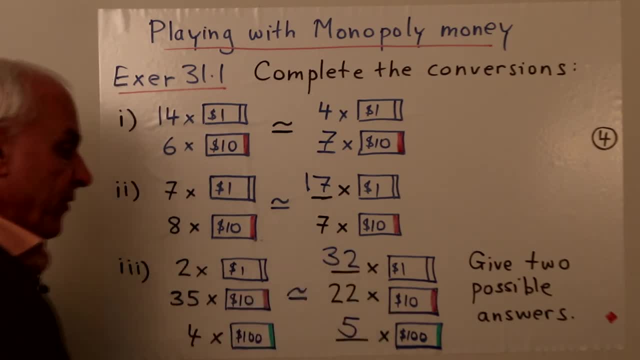 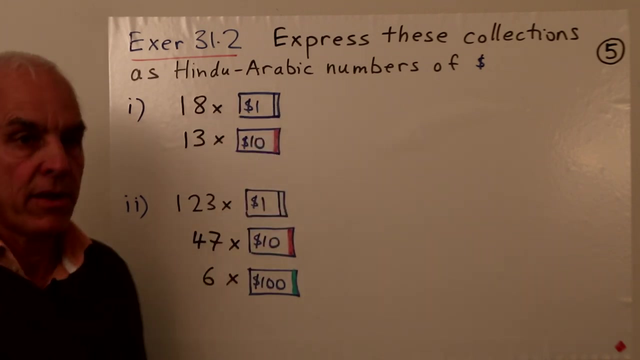 two one dollar bills, And now this is an equivalence. Now they represent the same amounts of money, even though the actual configurations are different. Now, in this exercise, we have to express these collections of money as Hindu-Arabic numbers of dollars. 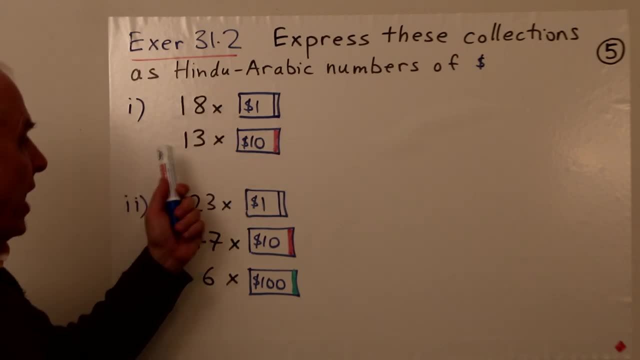 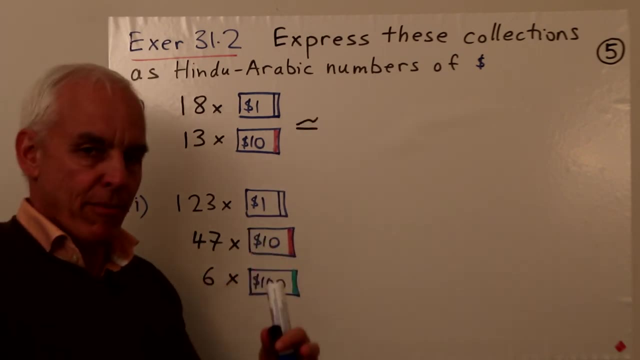 So here we have eighteen one dollar bills and thirteen ten dollar bills, And we want to find some equivalent open number first of all, that is like a Hindu-Arabic number, so that the number of bills is always at most nine. So what we have 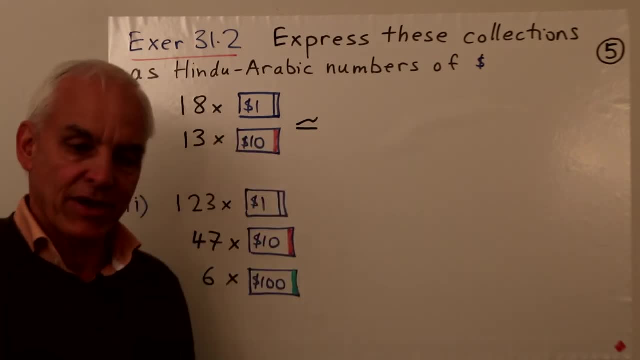 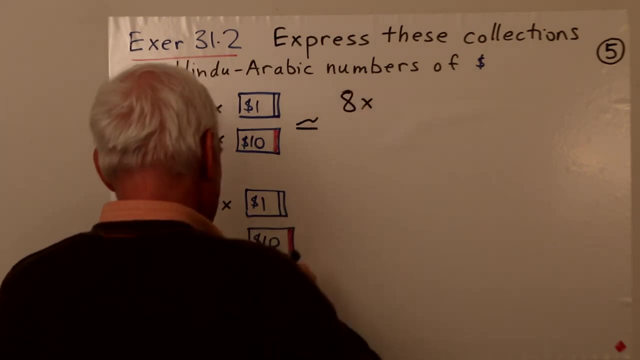 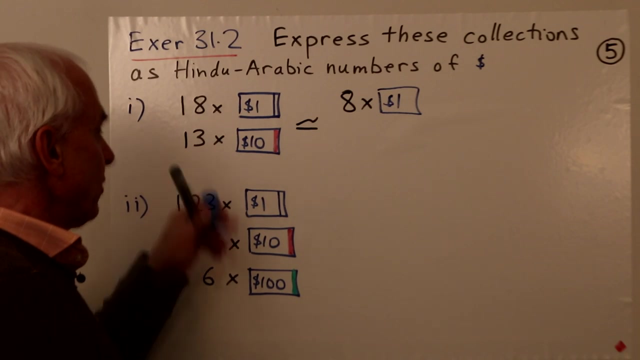 to do is we have to convert these eighteen one dollar bills into an amount less than or equal to nine. So that's meaning that we're going to take eight of them, So we have eight times one dollar, And ten of them will be converted into ten. 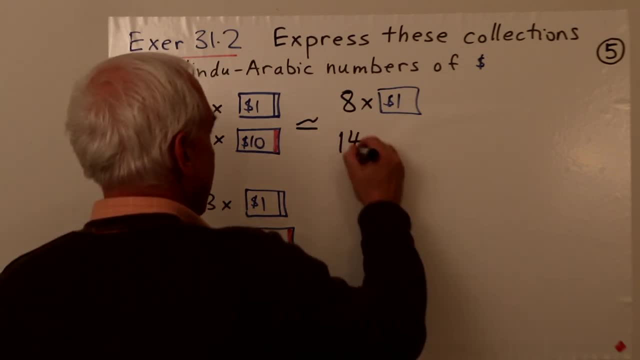 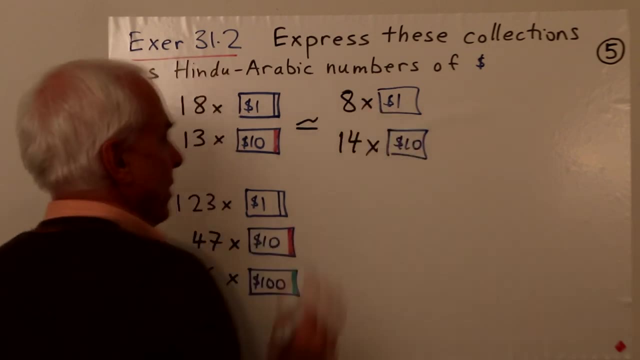 dollar bills. So I might just do it that way. So there's fourteen, ten dollar bills. Alright, that's sort of the first step. The first step. I've gotten the ones digit in the right range from zero to nine. Now the tens. 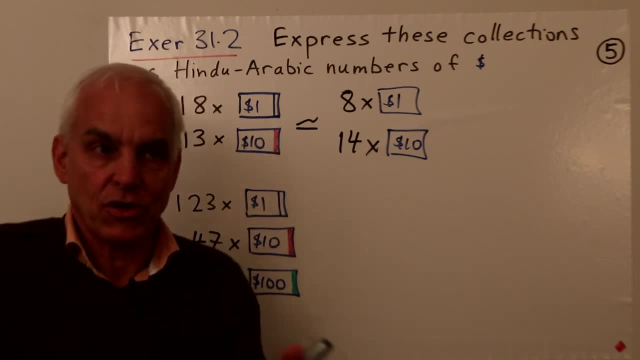 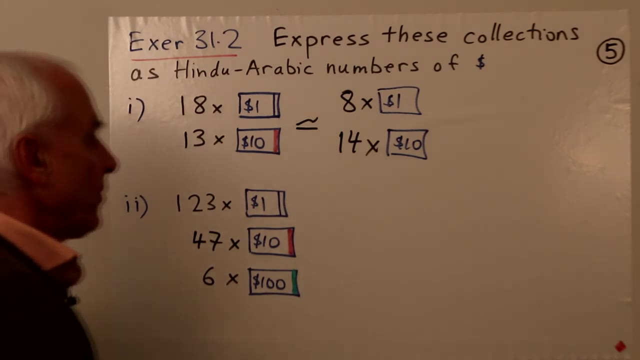 digit is still problematic because it's bigger than nine, So we have to convert it to something else. We have to get fewer than ten dollar bills. So how are we going to do that? Well, there'll still be eight times. I'll just 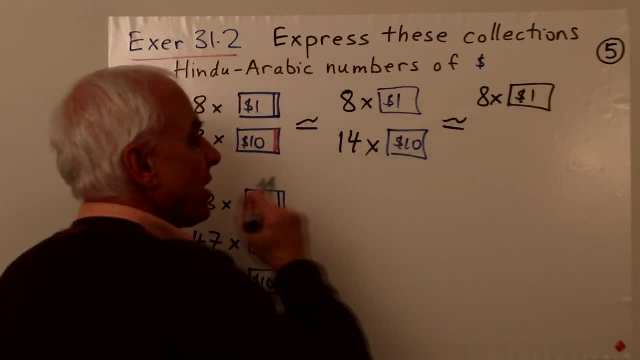 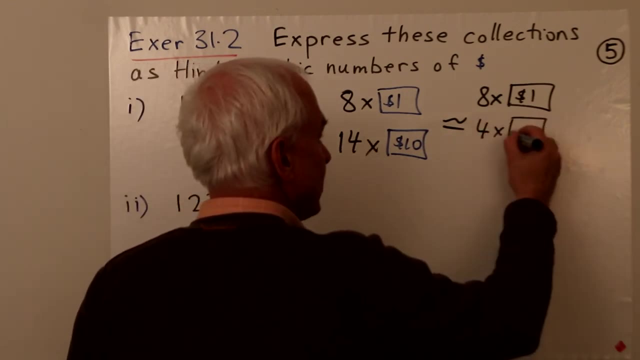 write like this: one dollar. And so I'm going to take ten of these ten dollar bills and convert them into a hundred, So that'll give me four times ten dollars, And ten of them will give me one times a hundred dollars. Okay, so I've made. 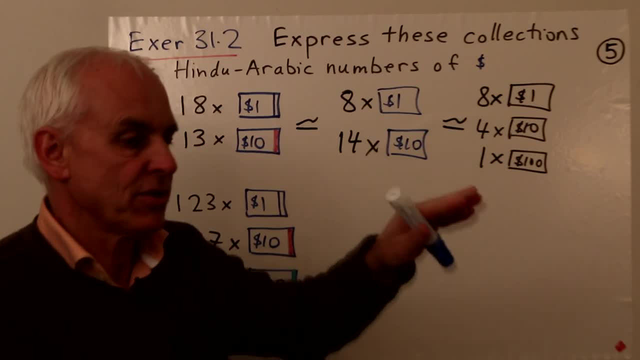 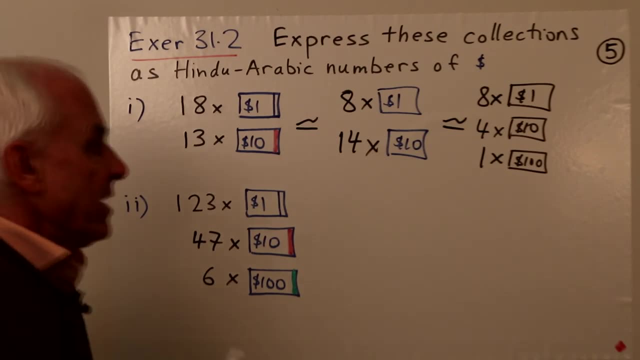 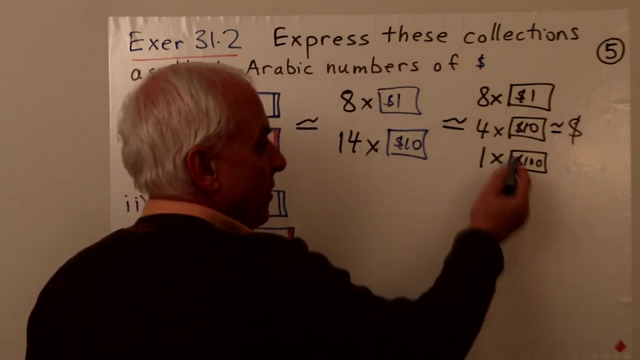 the conversion, And now all the coefficients, or all the quantities, or the digits are in the range zero to nine. So that's in Hindu Arabic form And I can write it in terms of dollars. It's a number that has one hundred four. 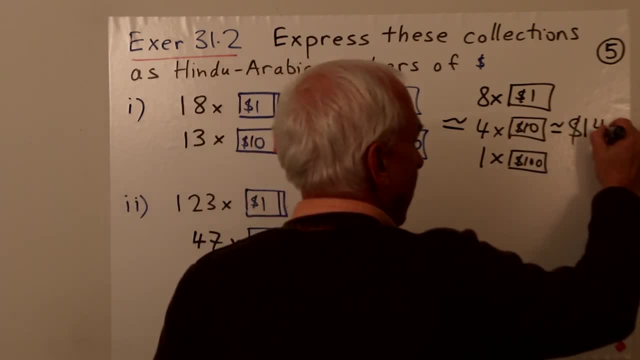 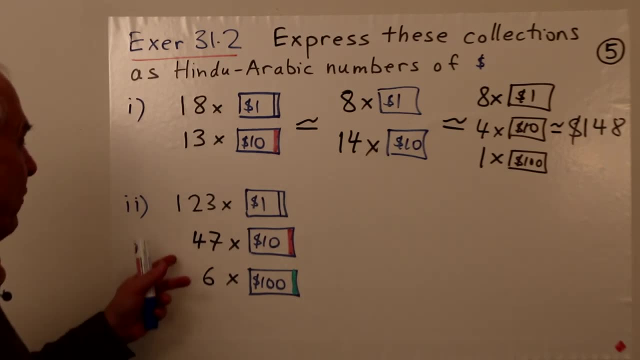 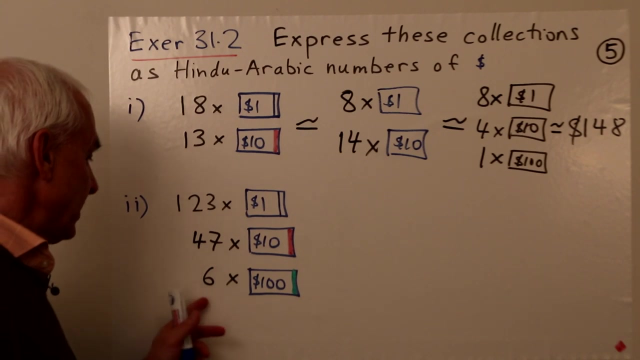 tens and eight ones, So it's one hundred and forty eight dollars. Okay, so let's have a look at this one: One hundred twenty three times one dollar, Forty seven times ten dollars And six times a hundred dollars. So we have to do a lot of converting. 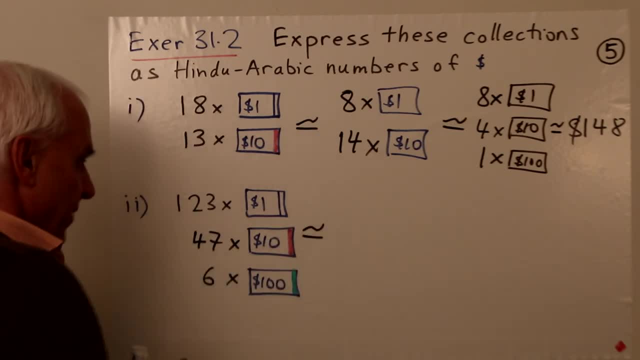 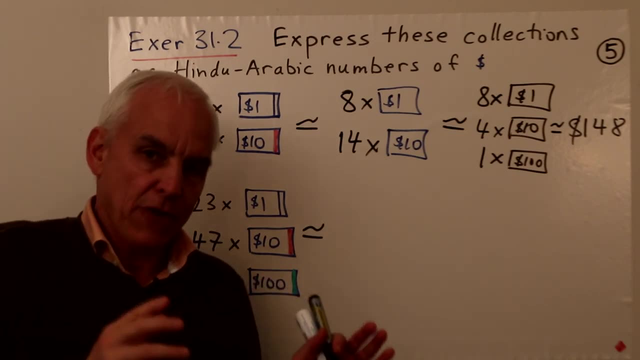 So we'll write the equivalent sign. And what are we going to do here? We have a hundred and twenty three one dollar bills. We're going to take a hundred and twenty of them and leave just three. So we'll leave three times one dollar. 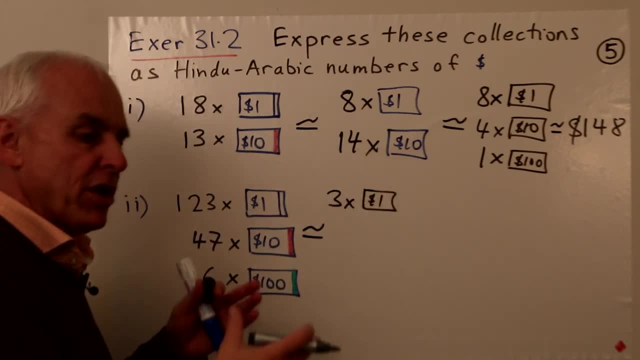 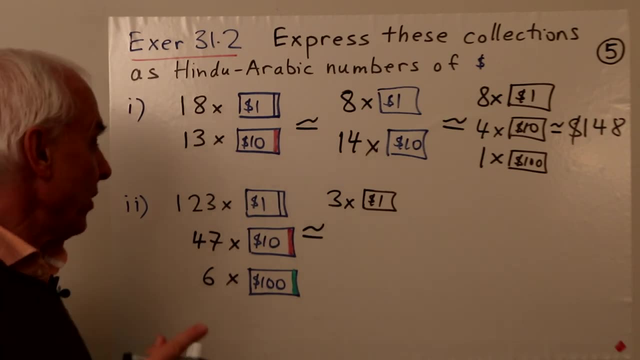 And the hundred and twenty of them we're going to convert to a hundred and twenty one dollar bills. It's the same as twelve ten dollar bills. So we're going to add twelve to what we already have. Okay, I'm going to suppose that we can add twelve. 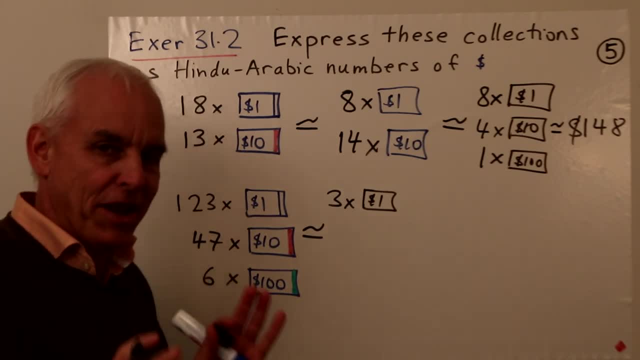 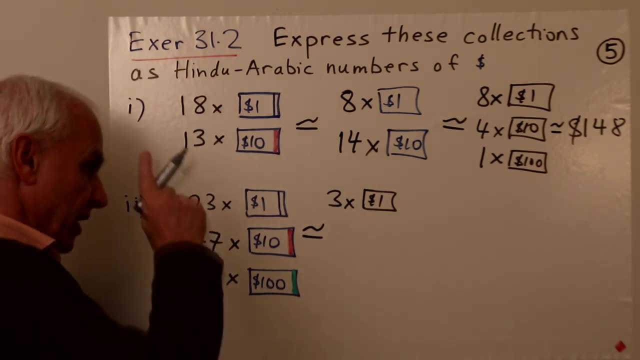 and forty seven. That might involve some thinking. At this stage we don't really know how to do a more complicated addition like that. very well, But okay, let's suppose we can do twelve plus forty seven, That's fifty nine, So we have. 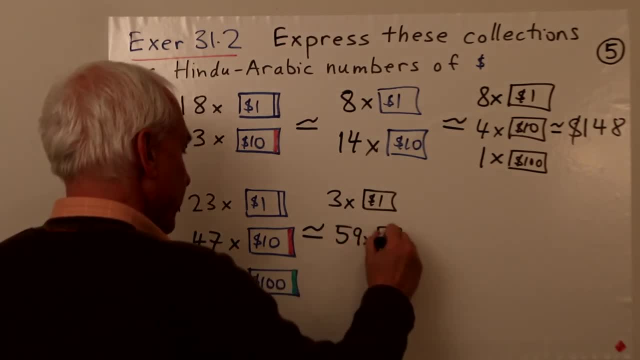 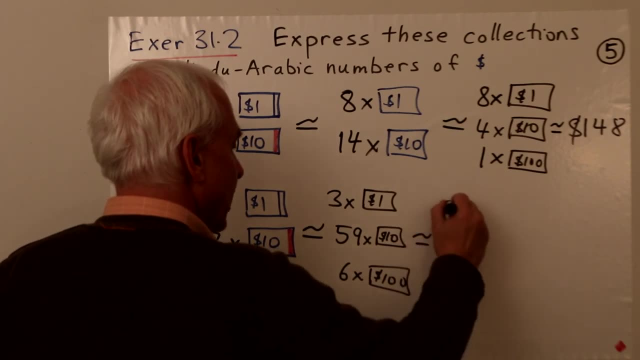 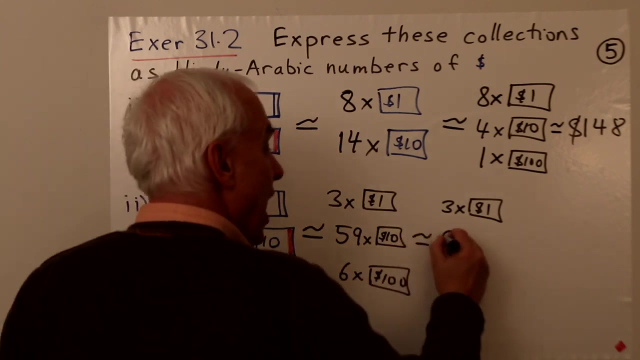 fifty nine, at this stage, times ten dollars, And still six times a hundred dollars. Okay, so now let's work. keep the three times ten dollars- Three times one dollar, rather- And the fifty nine times ten dollars. Well, that's going to become nine. 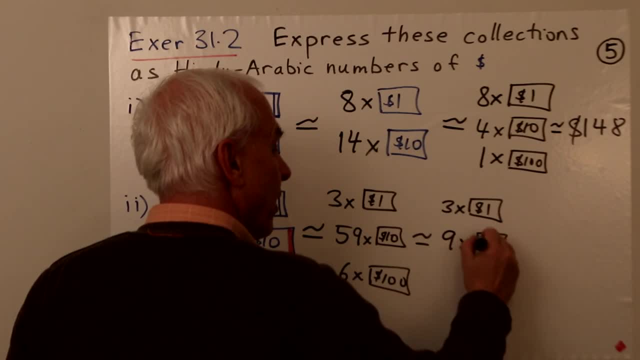 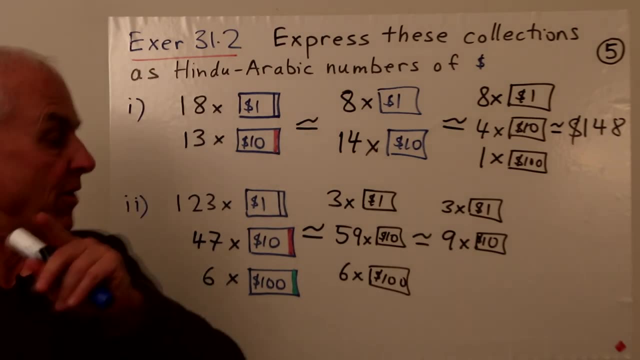 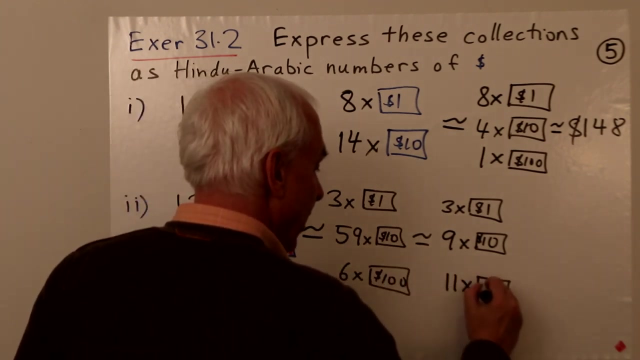 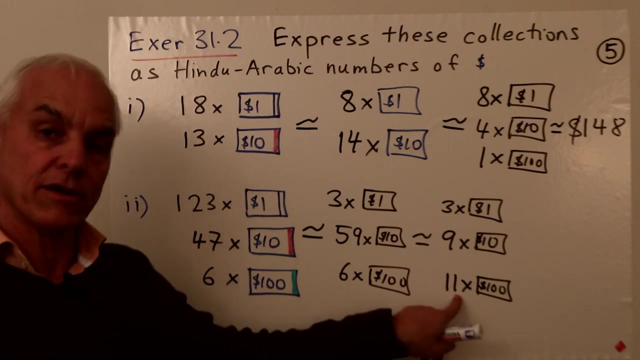 times ten dollars, And the fifty ten dollars is going to become five hundred dollars. So the five adds to the six and we get eleven times a hundred dollars. So that's almost finished, but not quite. That number is still bigger than nine, So we have to go. 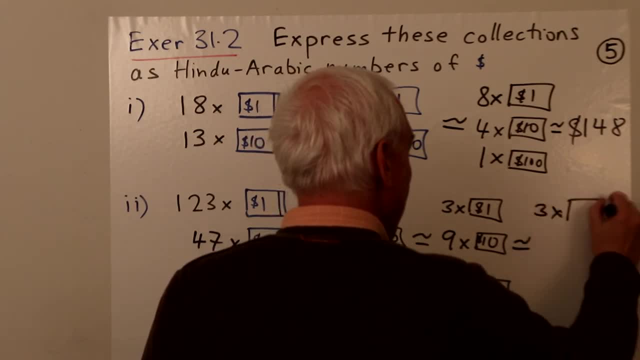 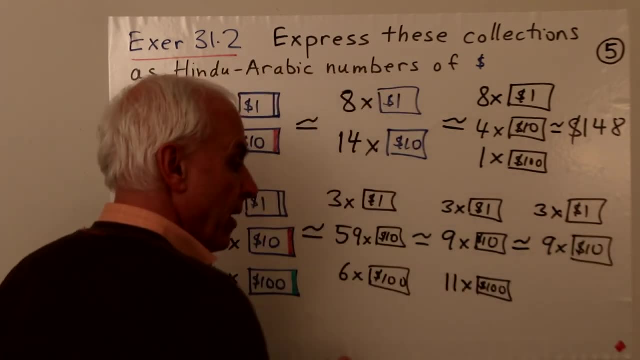 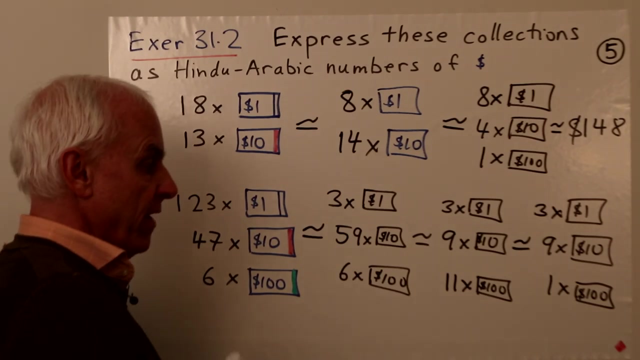 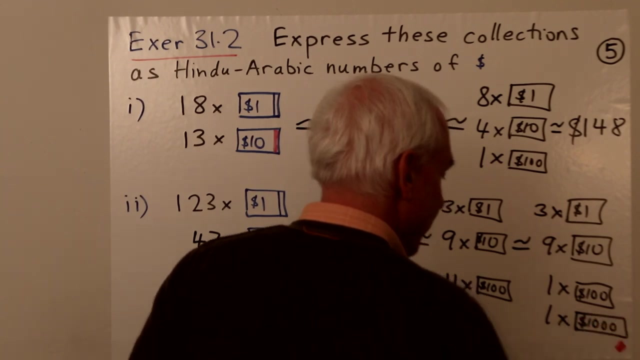 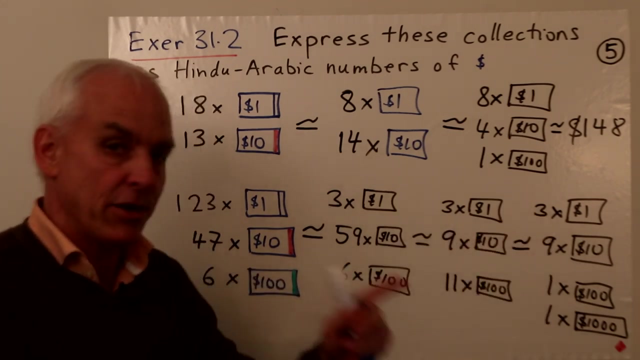 one more step: Three times one dollar, nine times ten dollars, And here we'll keep one of those hundreds And the other ten will peel off and convert into a single thousand, Alright, And at that stage we recognize a Hindu, Arabic number, because all the digits are less than or equal. 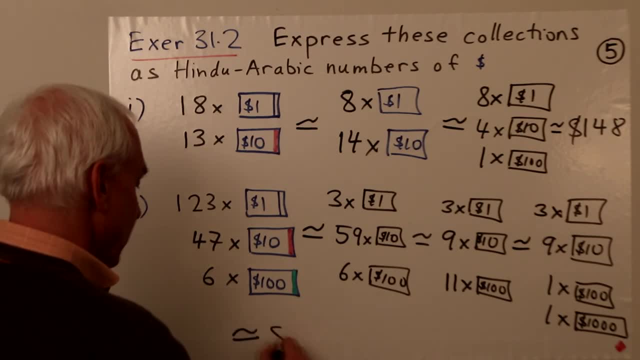 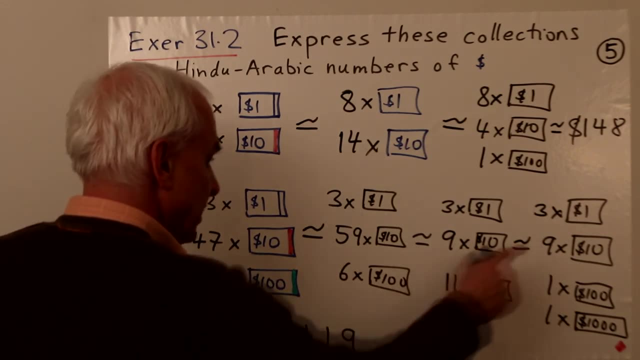 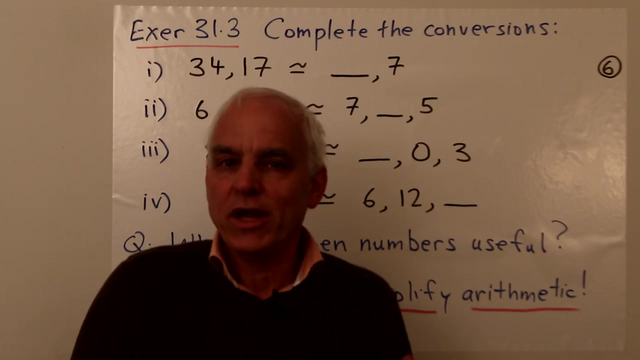 to nine. So the final answer down here in terms of dollars will be starting with the thousands One thousand one hundred ninety three. So, while our original motivation is coming from money, we can actually work with these open numbers purely independent of any monetary models. 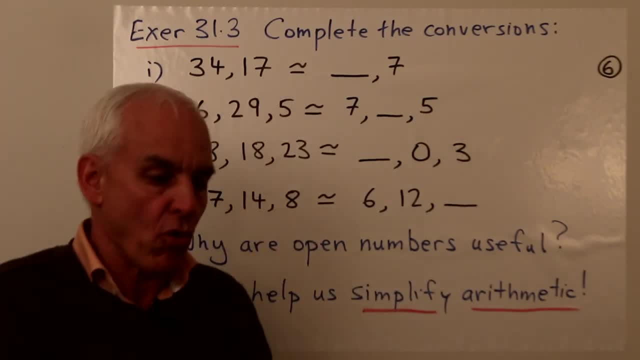 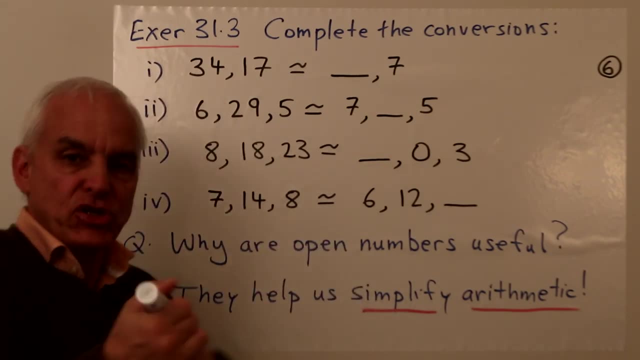 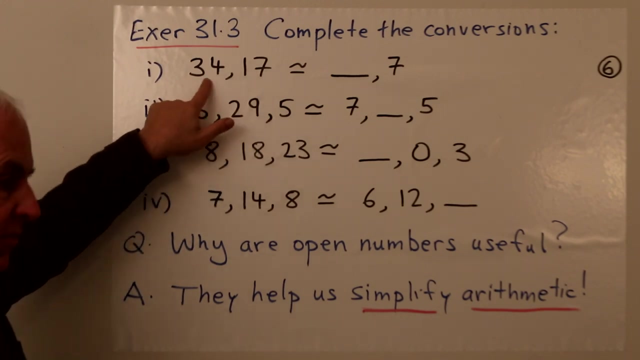 And this exercise just asks us to transform open numbers to equivalent open numbers, So to understand that process of exchange. So here we have thirty four, seventeen. The number of ones is the number of tens. We're converting it to some other open number where there are seven. 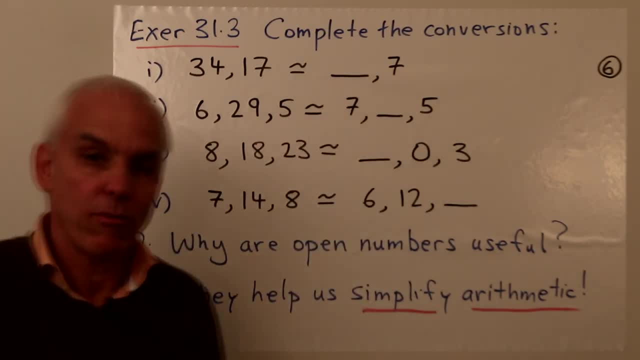 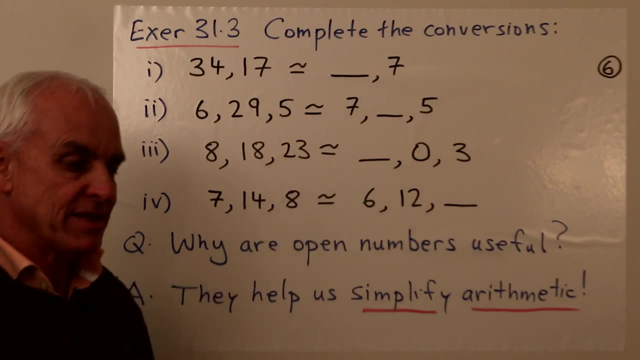 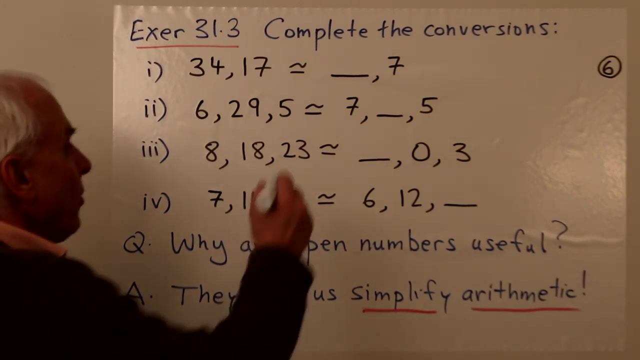 ones now And supposedly a certain number of tens. Well, there were seventeen ones here. There are seven ones here. That means ten of them have gone. They have been converted to a ten. So instead of having thirty four tens, we now have thirty five tens. 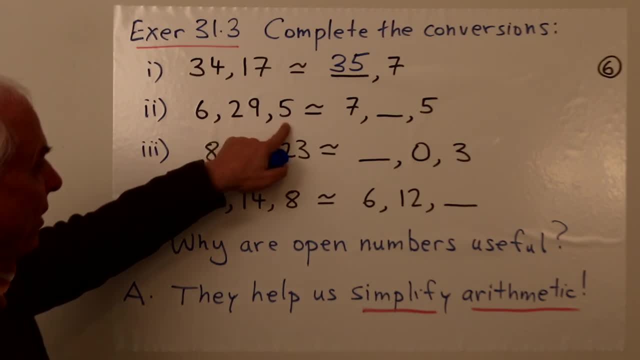 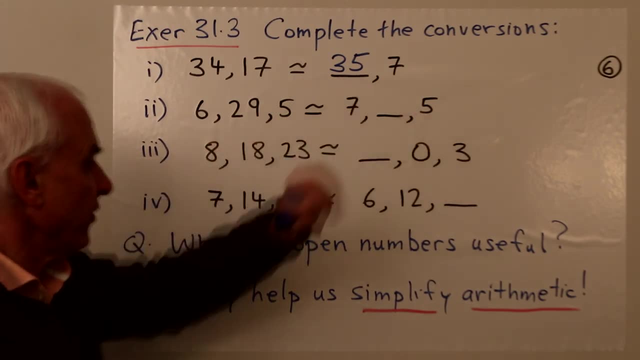 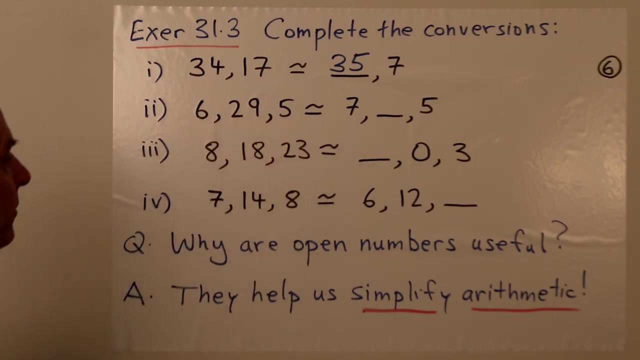 Here we have six twenty nine, five. We want to convert that to seven something five. Okay, what's different? The five is the same, The ones are the same, The hundreds have gone from six to seven. So how do we? 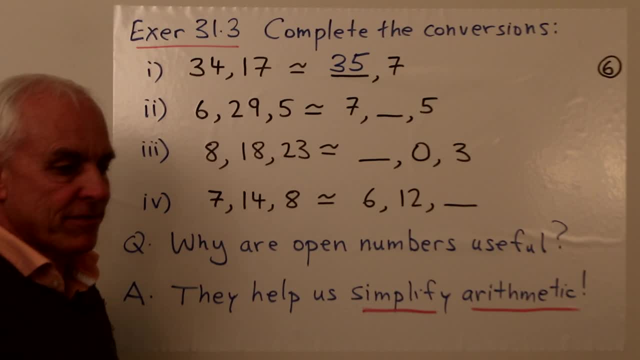 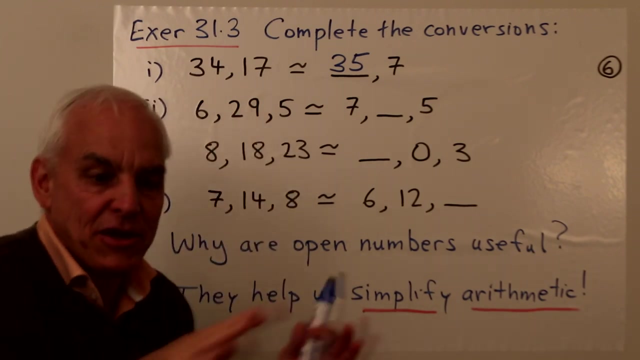 change from six hundreds to seven hundreds. It means we have to convert some of these tens to make a hundred. We need ten tens. We need to take ten of these twenty nine and convert them into a hundred. So when we do that, there will be 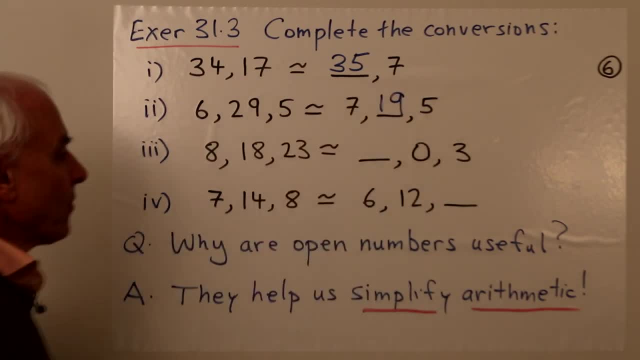 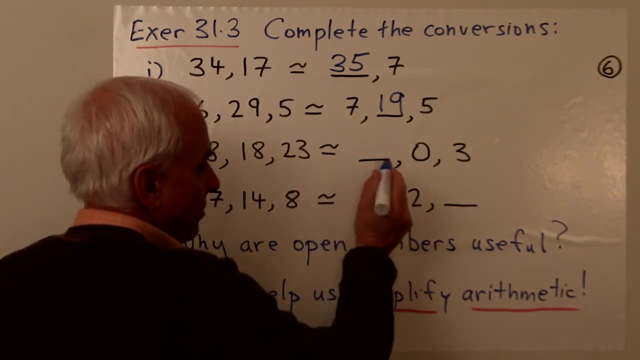 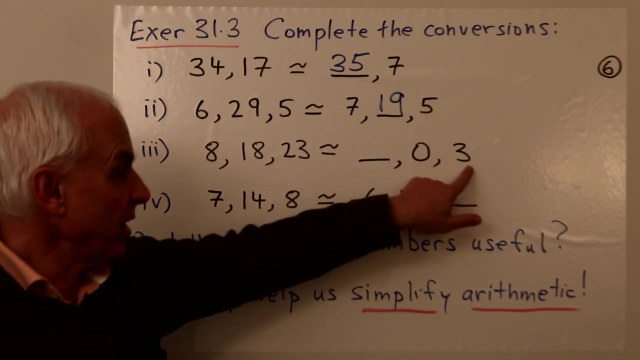 nineteen of them left Here. eight, eighteen, twenty three. We're converting it to something in the form blank zero, three, Zero three. Okay, there's three ones Here. there are twenty three ones, So we definitely have to get rid. 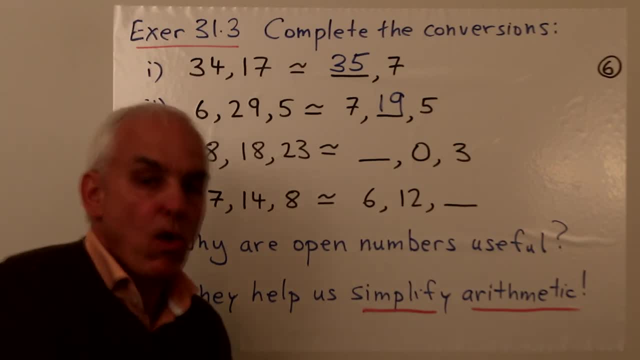 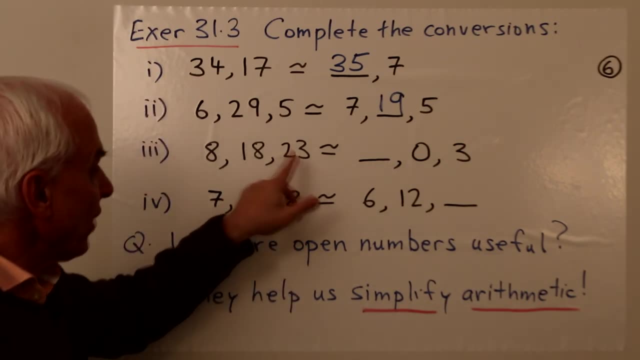 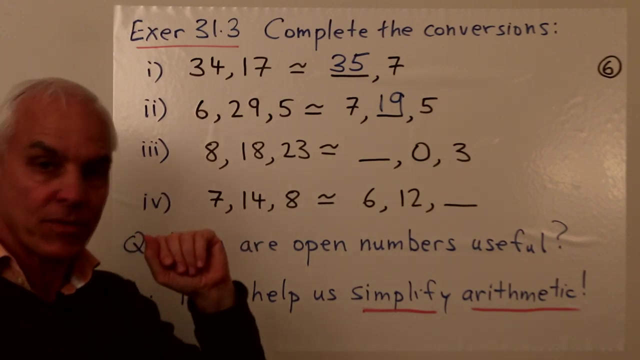 of twenty ones. Twenty ones converts to two tens. So we could change those twenty ones and convert it to two tens, making it all together twenty tens, Twenty tens over here, But over here we end up with only zero tens. That means that all 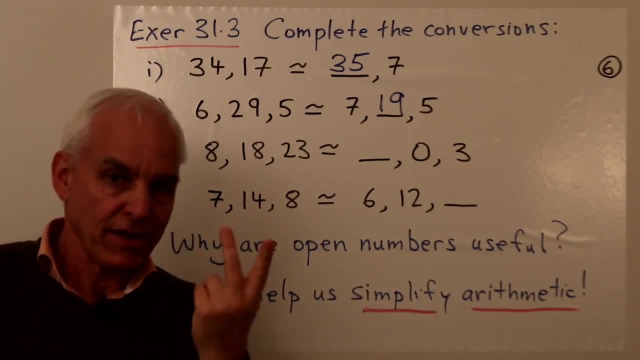 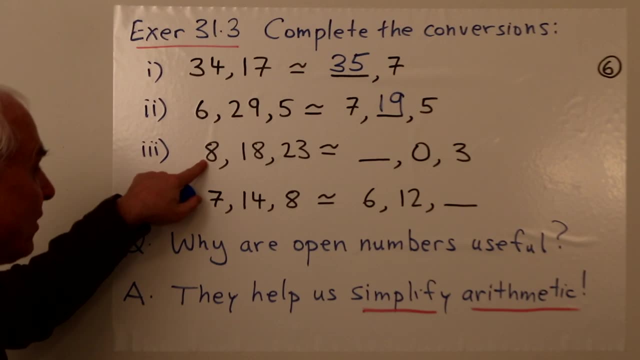 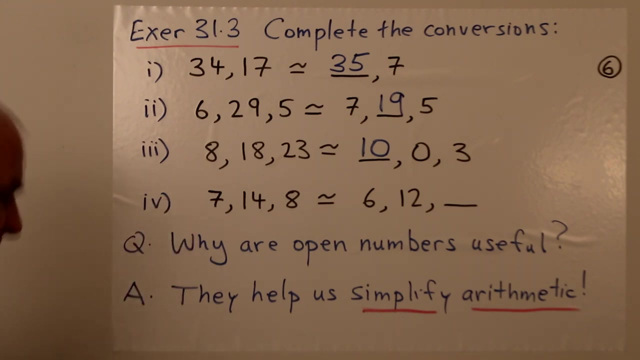 twenty tens were converted into hundreds. Twenty tens, well, ten tens make a hundred. so twenty tens is going to make two hundred. So we have to add two to eight. Okay, I'll let you figure out this one. Okay, so we have the rudiments. 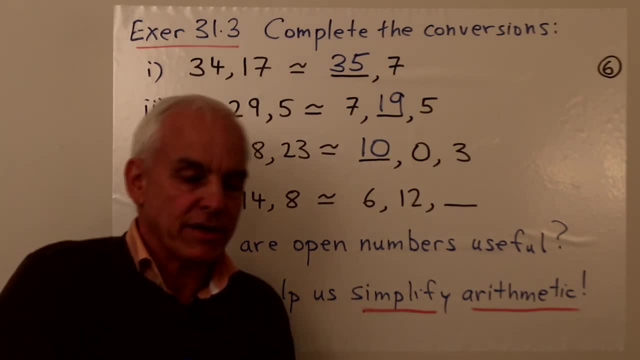 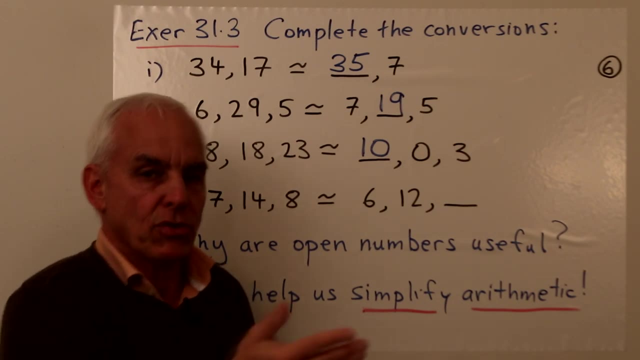 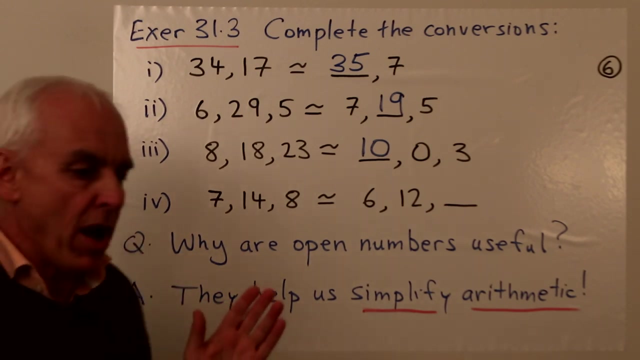 of when two open numbers are equivalent, How to sort of convert from one to the other and also how to sort of reduce an open number to some equivalent Hindu Arabic number. So we might ask now: why are open numbers useful? Why are we introducing this very 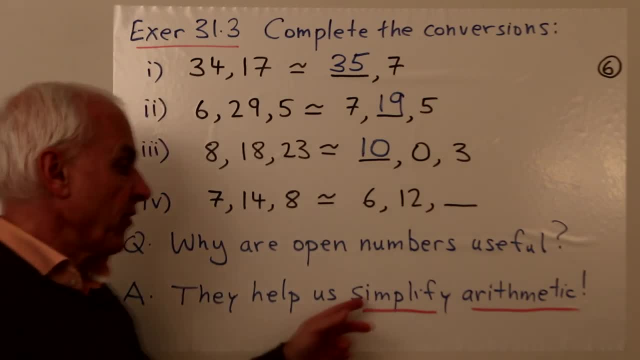 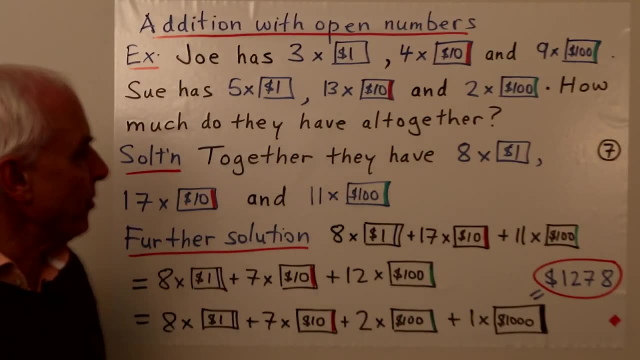 novel kind of arithmetic. And the answer is because they help us simplify arithmetic. So let's illustrate the potential application of open numbers to addition with this example: Joe has three one dollar bills, four ten dollar bills and nine hundred dollar bills, While 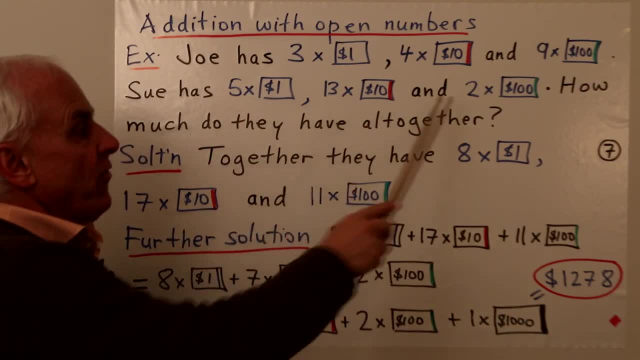 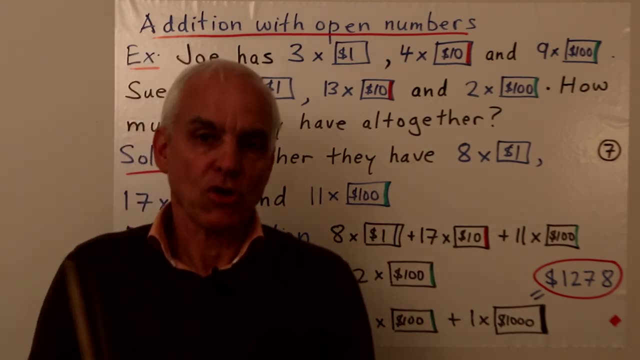 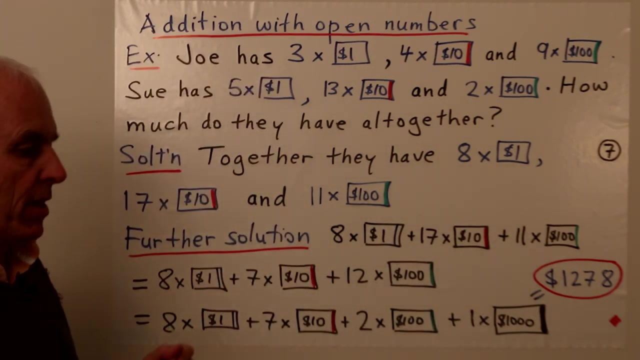 Sue has five one dollar bills, thirteen ten dollar bills and two hundred dollar bills. How much do they have all together? So combining their monies? So the first solution Together means we're putting everything in one pile, So we just do everything. 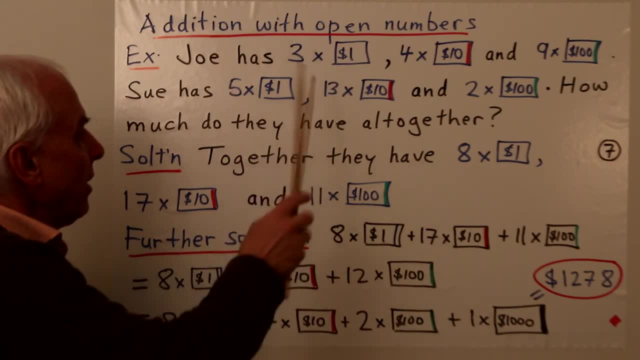 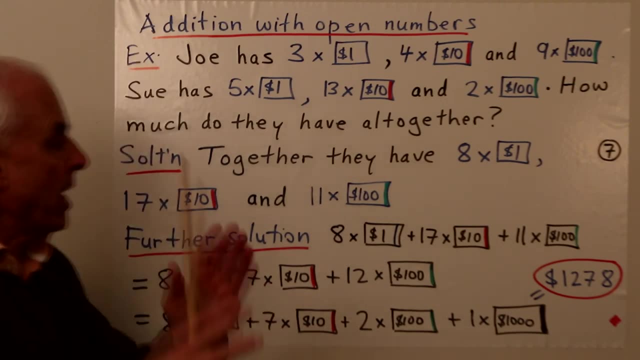 individually. We look at the one dollars. Joe has three, Sue has five. Together they have eight. So together they have eight one dollar bills. And now we look at the ten dollar bills. Joe has four, Sue has thirteen, Four plus. 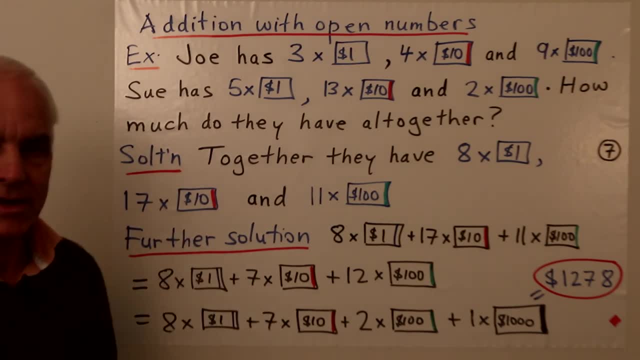 thirteen is seventeen, So together they have seventeen ten dollar bills. Nine hundred dollar bills has Joe, Two hundred dollar bills has Sue. All together that's eleven hundred dollar bills. So if they combined their monies, this is an accurate description of what they would have. 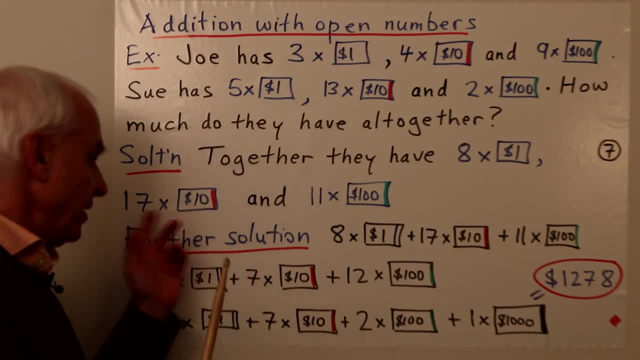 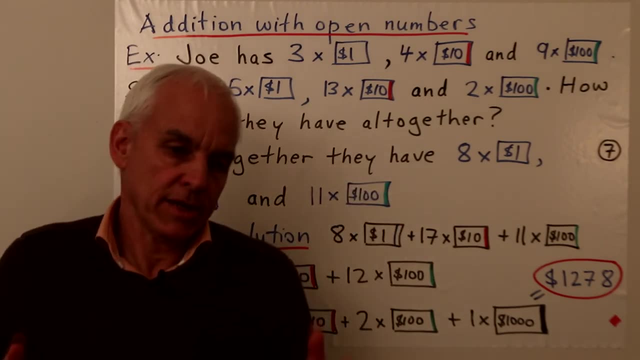 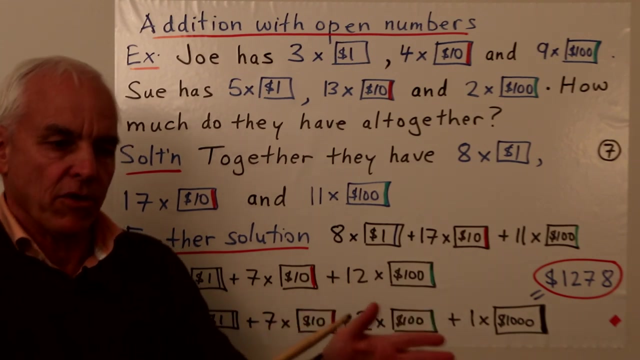 They would have eight one dollar bills, Seventeen ten dollar bills And eleven hundred dollar bills. That is in some sense a reasonable solution, But it's also possible that the intent of the question was maybe a little bit further. Maybe the question was actually asking: 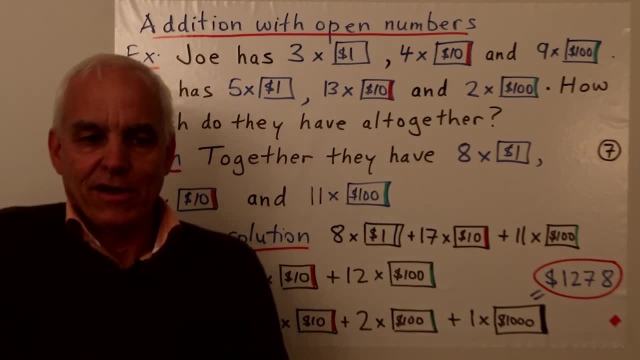 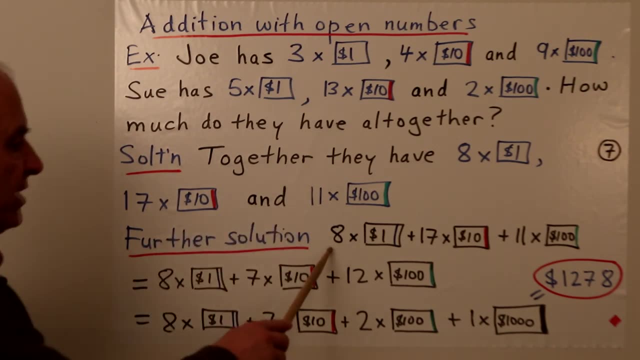 how much money do they have in kind of a usual sense? So let's go a little bit further and see what happens. Here's eight one dollar bills, Seventeen ten dollar bills And eleven hundred dollar bills. What happens when we add all of that together? 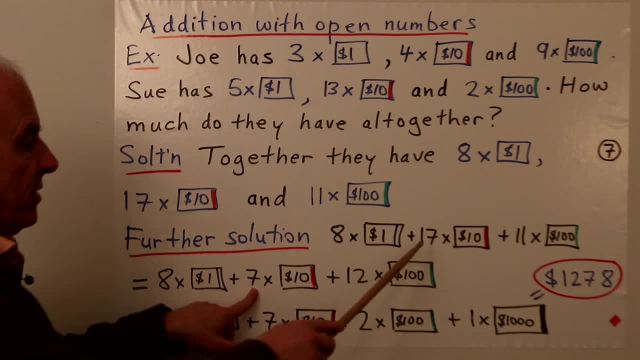 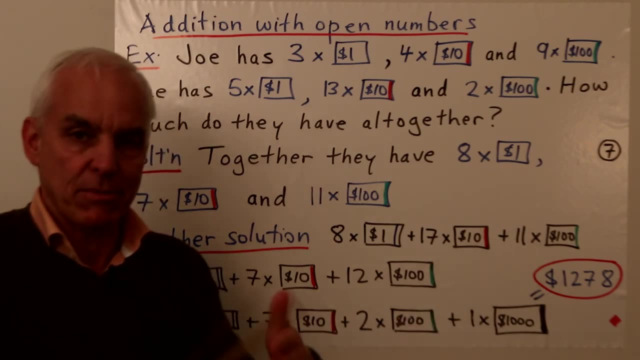 So here's eight one dollar bills. We're going to convert the seventeen ten dollar bills to seven ten dollar bills and twelve hundred dollar bills. Exactly the same kind of thing that we've been doing, And now it's almost in Hindu Arabic form, except there's a twelve here. 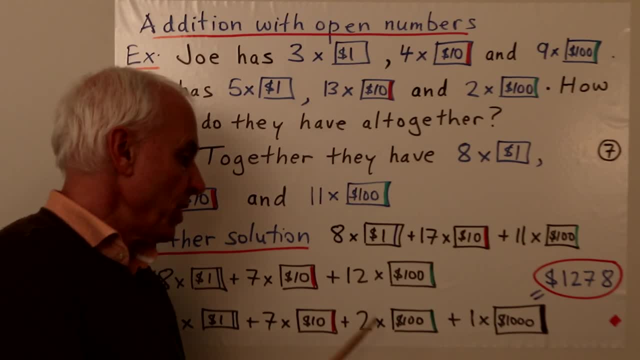 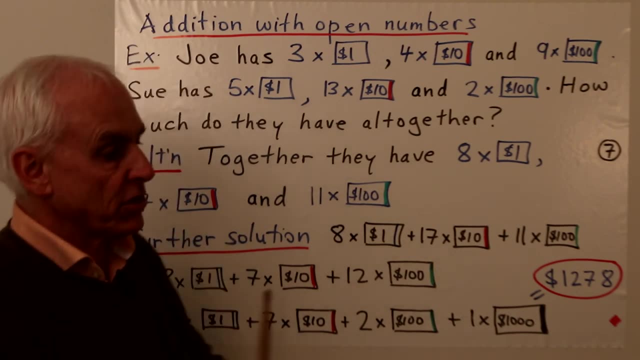 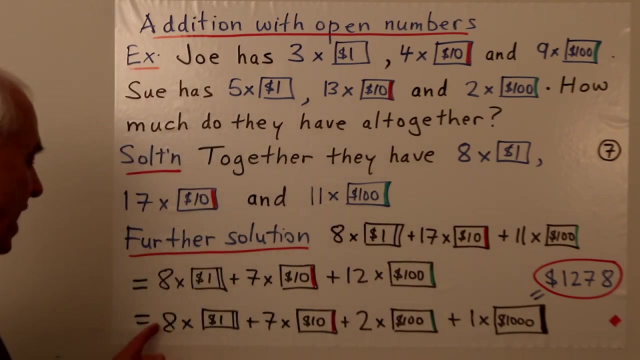 So we keep the eight, one dollar bills, We keep the seven, ten dollar bills. So we take two of those hundred dollar bills and keep them where they are, And the other ten we convert to a thousand dollar bill. So one thousand dollar bill, And now it's in. 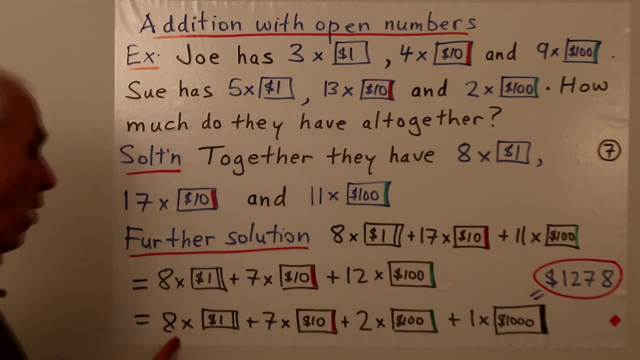 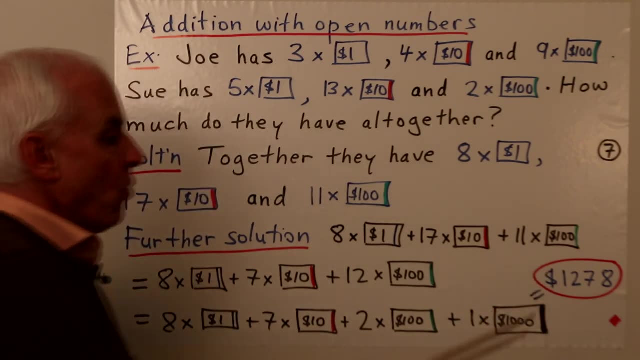 Hindu Arabic form with an eight, a seven, a two and a one, Starting with the ones, and then the tens, and then the hundreds and then the thousand, And so we can write it in the standard Hindu Arabic form as one thousand two hundred and seventy eight. 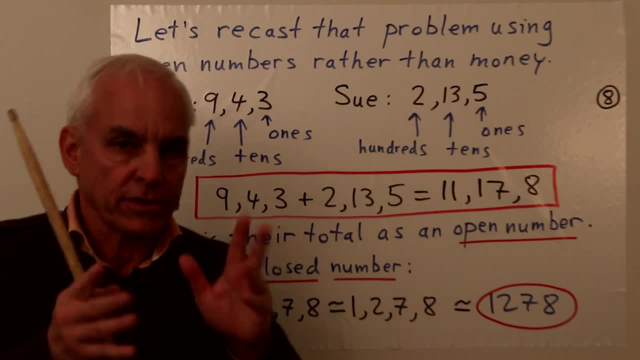 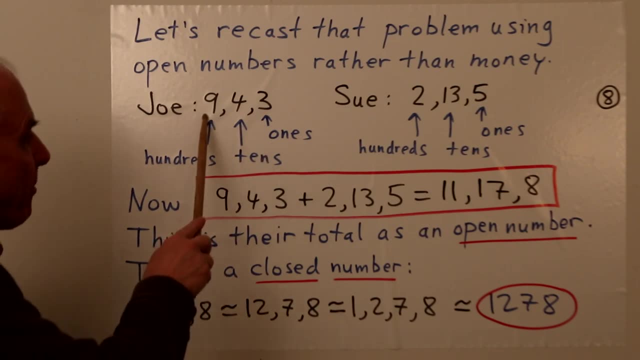 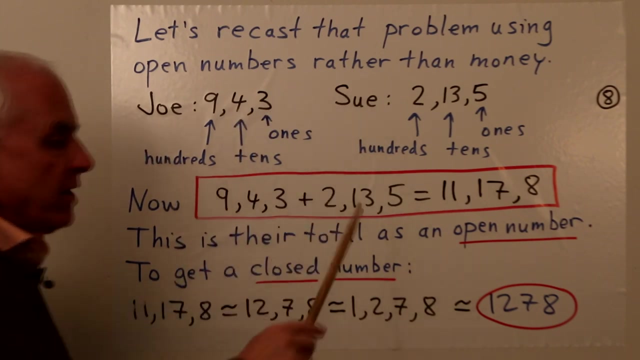 dollars. So let's state that problem without lots of dollar bill pictures. Joe has money which is represented by the open number nine, four, three Ones, tens, hundreds. Sue has money represented by the open number two, thirteen, five, Five ones, thirteen. 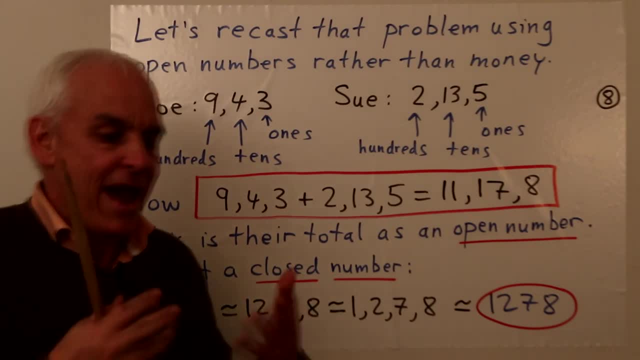 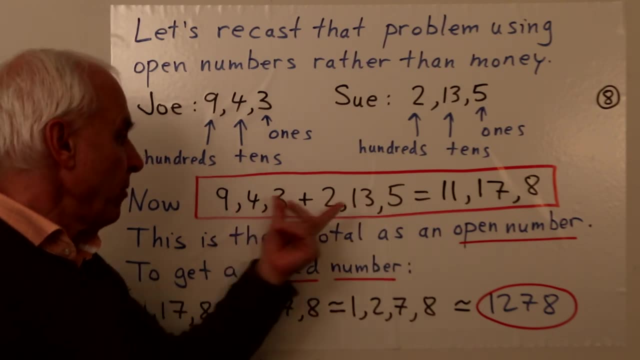 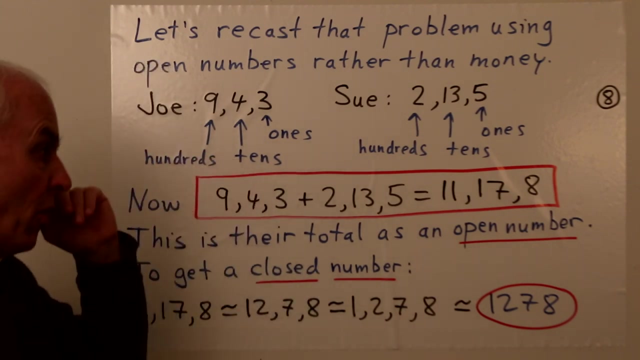 tens and two hundreds. When we want to add their monies, we're adding these two open numbers: Nine, four, three plus two thirteen, five. How do we do that? Well, what we did, in sort of the first solution, was we just added the ones. 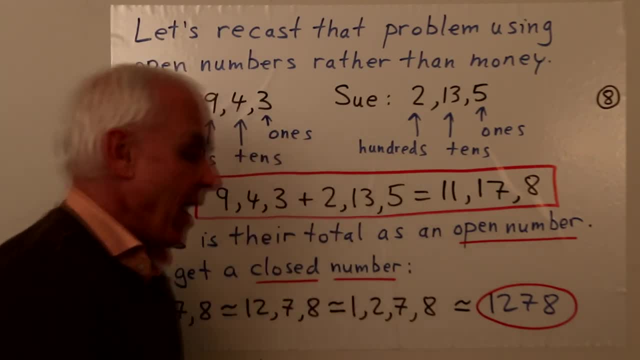 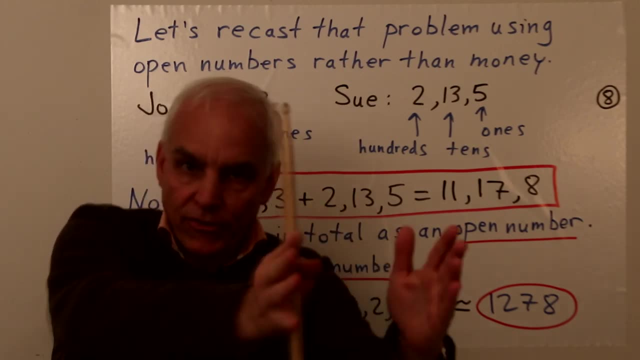 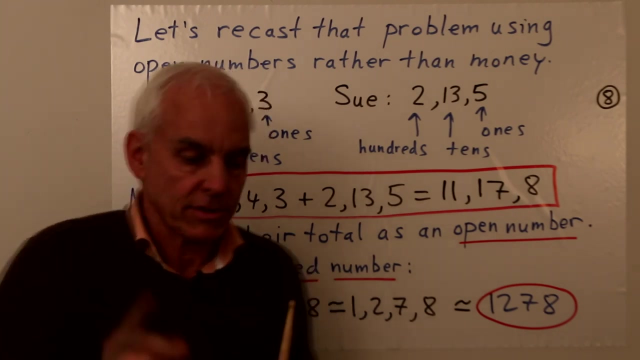 we added the tens and we added the hundreds And there was no interaction between those three. They were each in their own lane like swimmers: No moving from one lane to another, No worrying about carryings. That's the beauty of this. So the three 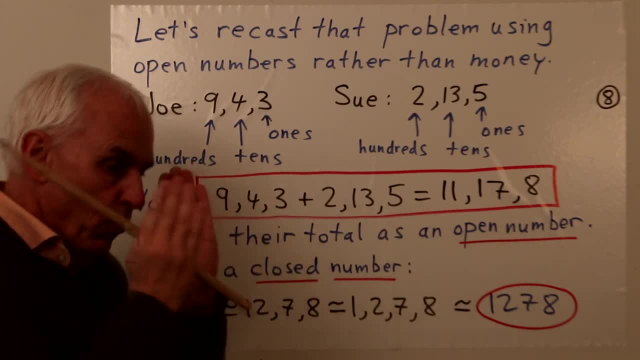 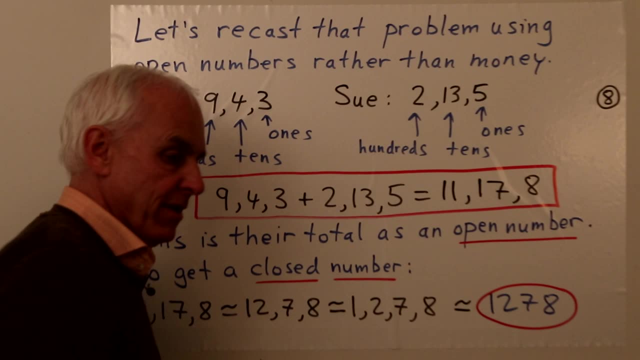 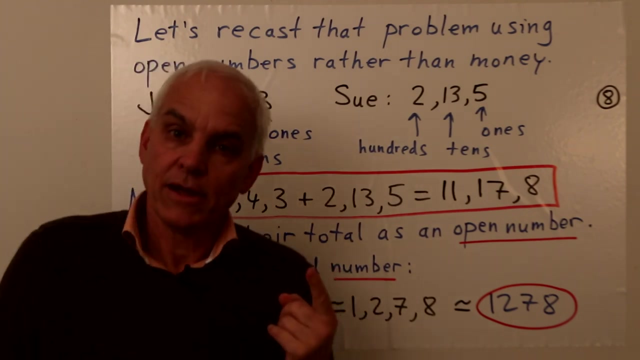 plus five is eight. That's a calculation purely in the tens digit. In the tens digit there's four and thirteen. Four plus thirteen is seventeen. In the hundreds, nine plus two is eleven. So you can see that addition with open numbers is going to be. 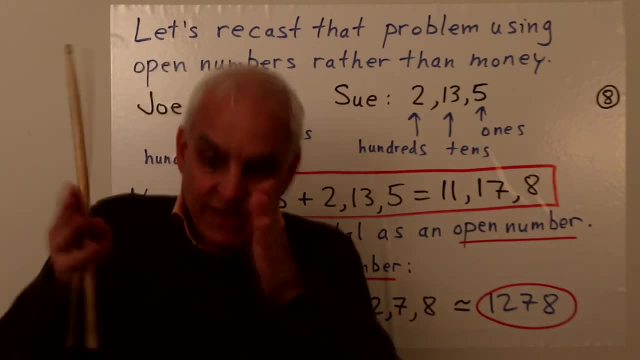 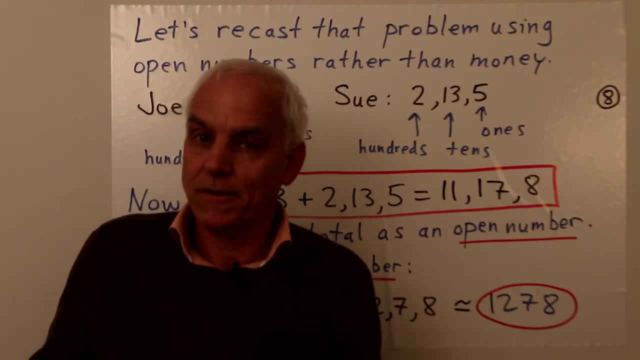 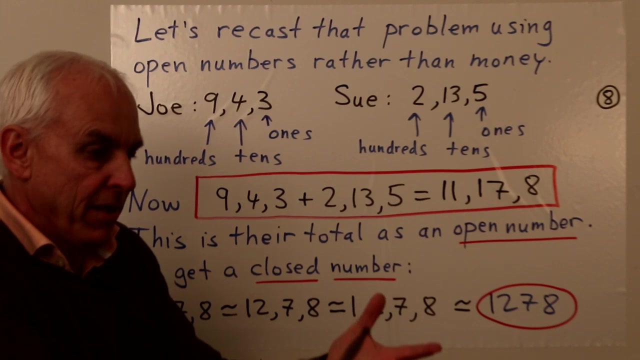 simple, because we're just going to keep each of the digits separate. The commas are separating things and there's no interaction between these things. There doesn't have to be Now. this is their total. as an open number. It actually reflects physically what they would have when they pool. 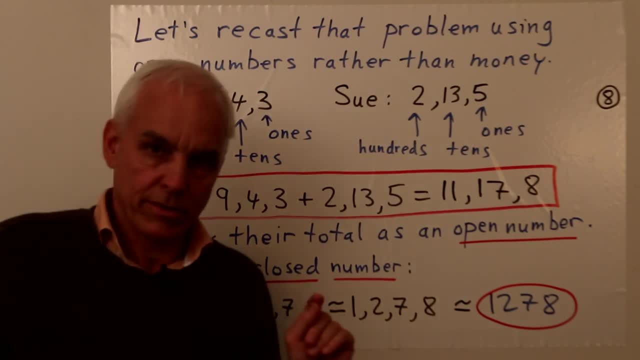 their money, But to get a closed number, which is maybe a term that we'll use to represent a Hindu Arabic number, A closed number as opposed to open number. What we want to do is we want to take this eleven, seventeen and eight, and 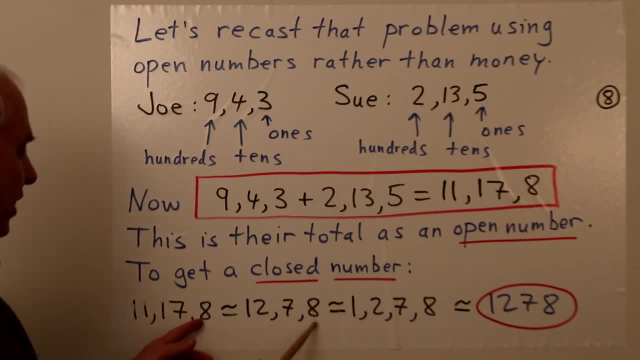 convert it. Okay, the eight stays where it is, The seventeen becomes seven, and ten of those get transferred to a hundred, So the eleven becomes a twelve, And then, at the next stage, the eight and the seven stay where they are, And the twelve well. 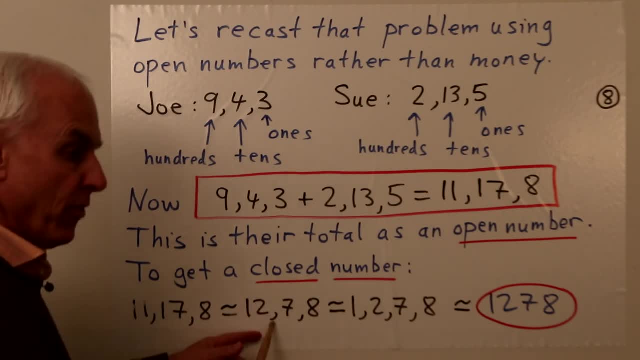 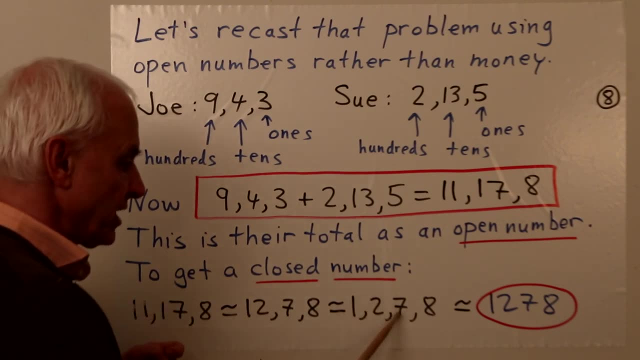 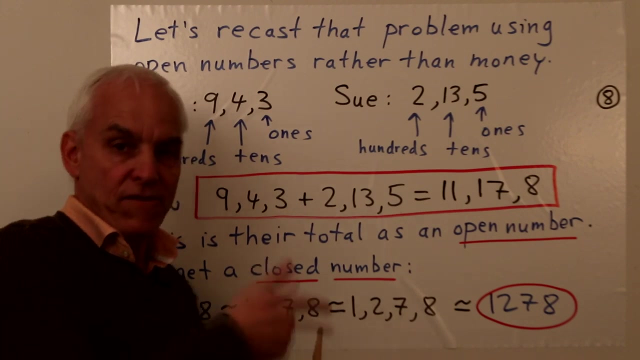 the two stays where it is, And ten of these hundreds are converted to a single thousand. So at this stage, one, two, seven, eight- all the digits are less than or equal to nine. We recognize aha. that's then in the form of: 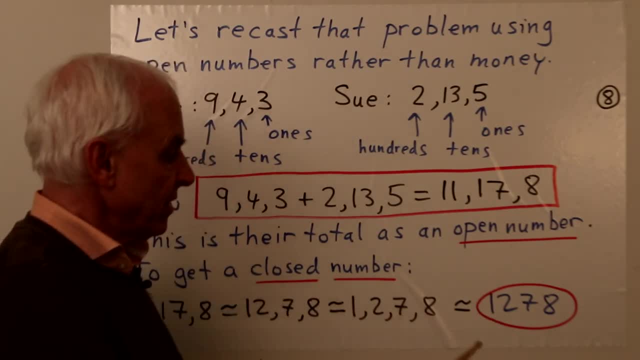 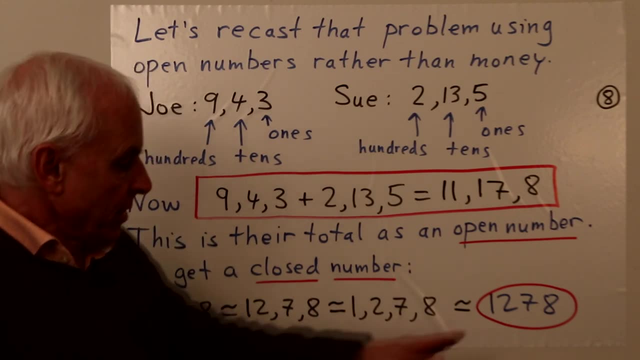 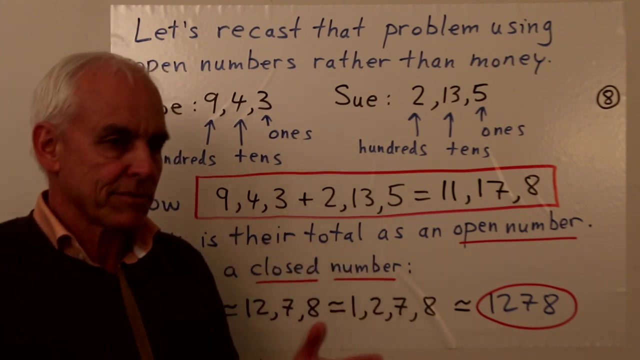 a Hindu Arabic number And then we can write it as equivalent to this Hindu Arabic number: One, two, seven, eight, without any commas. So this is a Hindu Arabic number, or maybe a closed number. It's final. There's no alternate formulations. 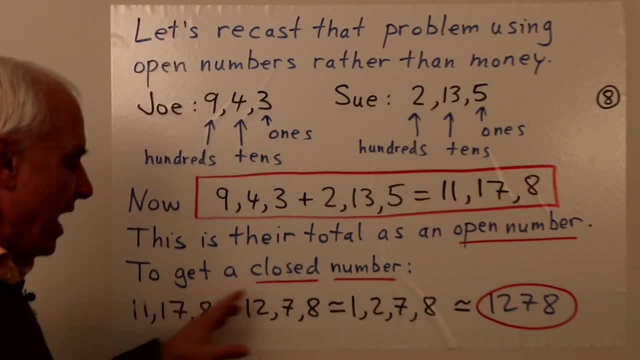 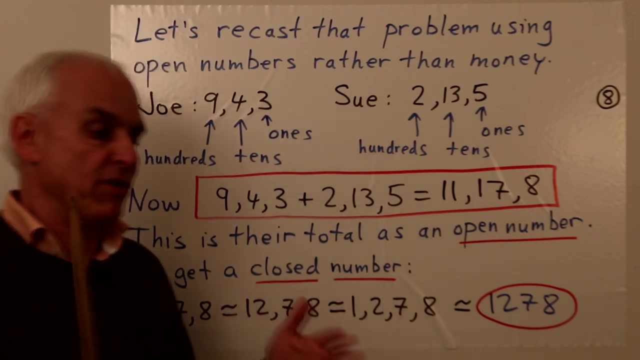 It's unique. The flexibility that we had with the open numbers is gone, Which is good, but also sometimes a bit of a disadvantage. Okay, so this corresponds to what I just did on the previous slide, but without any pictures, without any reference to the 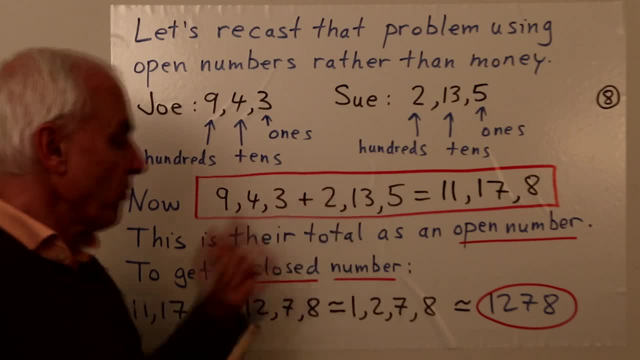 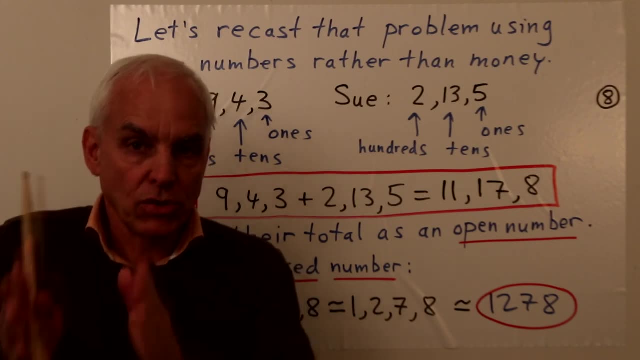 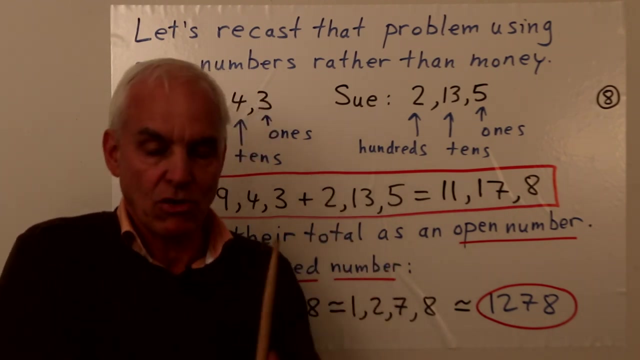 dollar bills and ten dollar bills and so on. We're really just doing arithmetic with open numbers here, And the crucial thing to remember is that we are just treating each unit separately. The ones are treated separately, the tens are treated separately, the hundreds are treated separately, and so on. 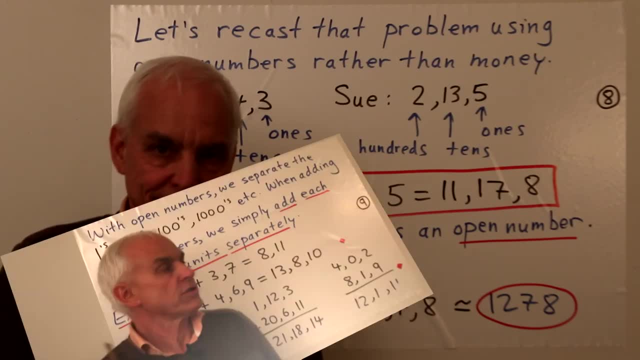 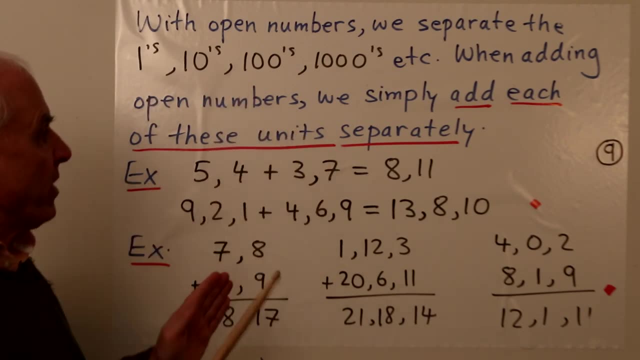 Everything stays in its lane. Okay, so what I've just said is that with open numbers, we separate the ones, the tens, the hundreds, the thousands, etc. And when adding open numbers, we simply add each of these units separately. Okay, so the commas are. 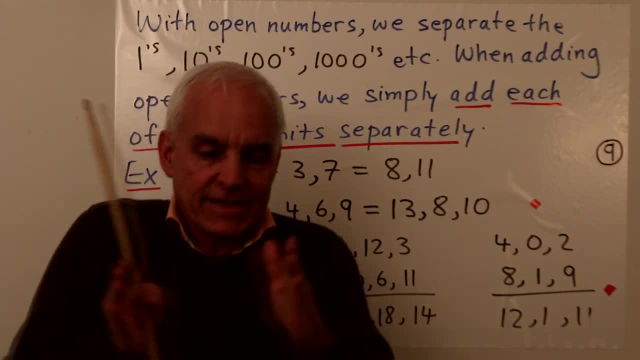 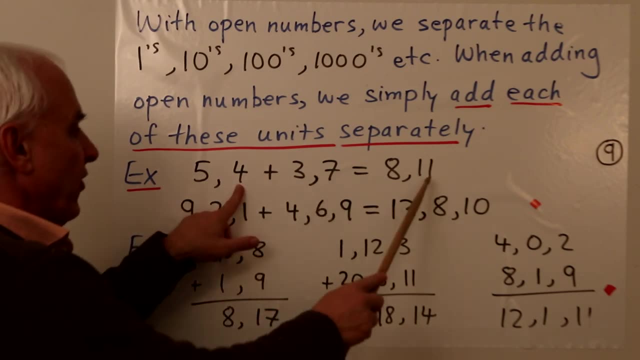 separating these things and we really want to maintain this separation between these various units. So, for example, five, four plus three, seven, We add the ones. we add the tens. Nine, two, one plus four, six, nine, We add the ones. 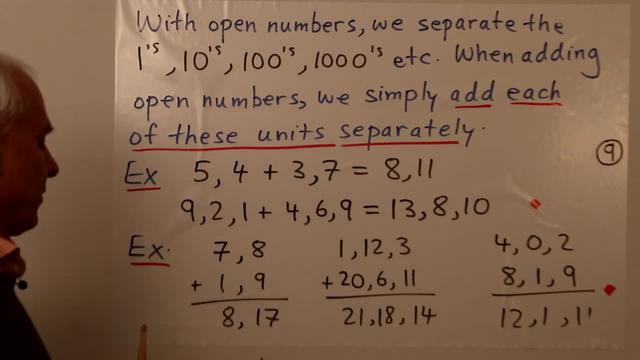 we add the tens, we add the hundreds, We can also arrange things vertically, And when we're adding more numbers, that's actually a very useful thing to do. So seven, eight plus one, nine, It's the same kind of thing. 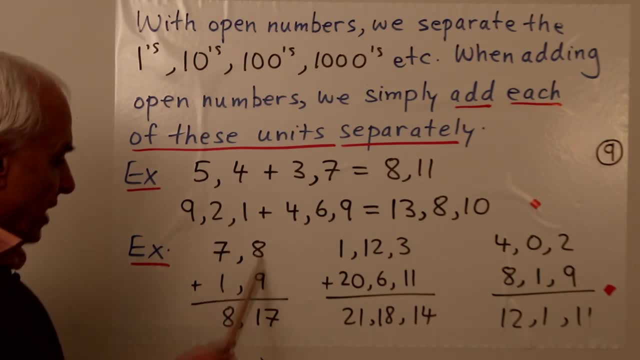 as this, except that we're writing it vertically. The ones are now aligned here on the right. It's very easy to add them up because they're on top of each other. So eight plus nine is seventeen. Here are the tens on top of each other.